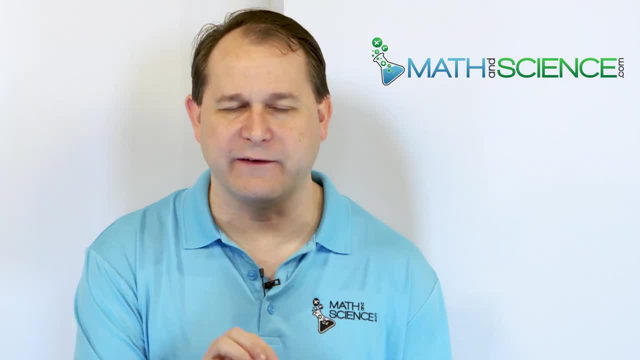 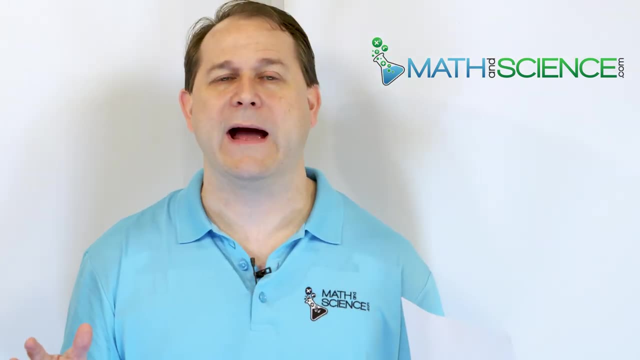 has, And so just to kind of let you know where the name of this person comes from. he's extremely famous and invented lots and lots of things when it comes to also algebra and also higher level math. In fact, when you think of the XY plane, you know the XY plane we use for. 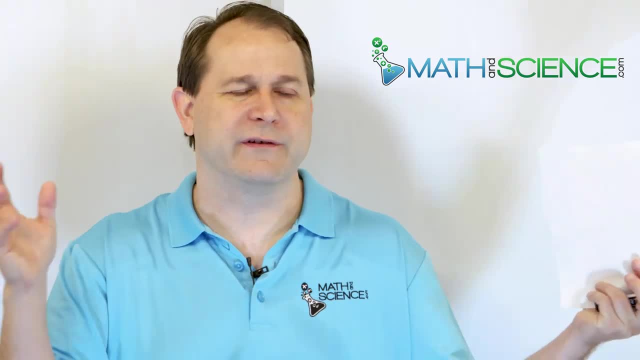 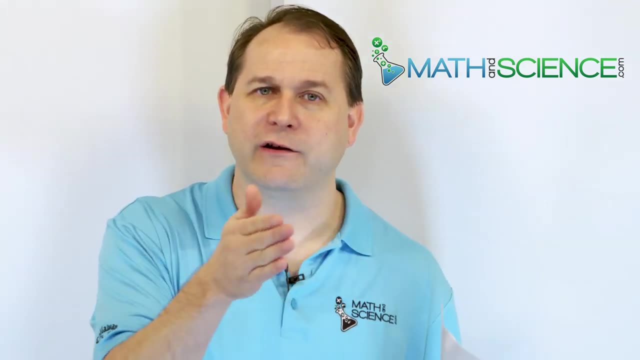 everything from plotting functions, plotting lines, plotting circles and ellipses. later on, The XY plane is actually called the Cartesian plane, from Descartes Descartes- Cartesian, that's where it comes from. So he invented lots of very useful things, And when working on these, 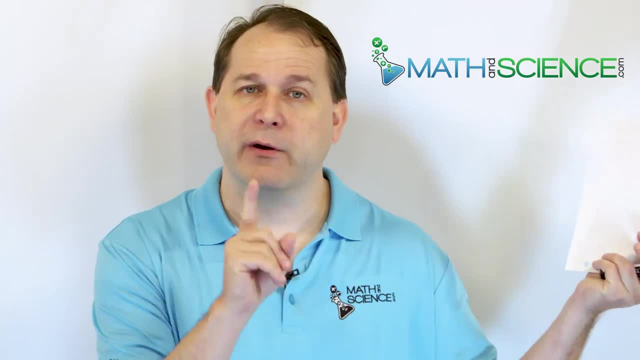 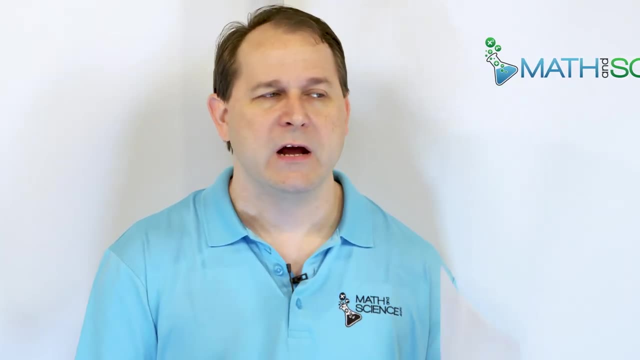 polynomials. now you know that we have a polynomial of first order: is a line. We know how many roots a line has. We know how to solve pretty much all lines. So we know how to solve all lines To figure out their roots. We know how to solve quadratics. Those are a degree of two, We know. 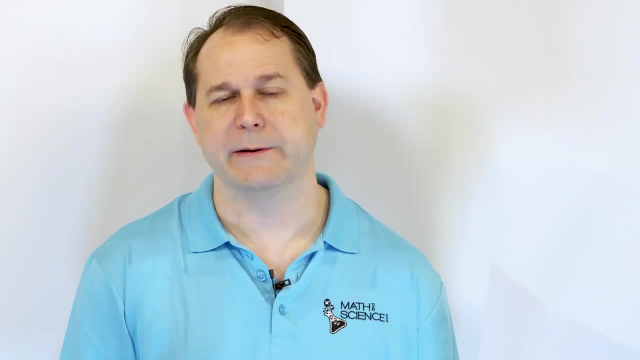 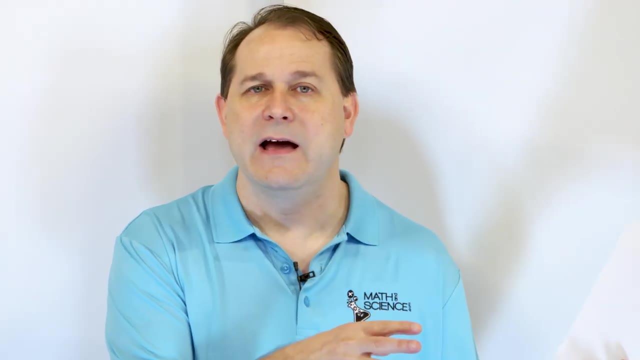 how to factor them. And if we can't factor them, we can always use the quadratic formula for roots of three and four and higher. Things get a little bit more difficult. We can sometimes do it by guessing one of the roots and then using division to find the other two roots. But when the 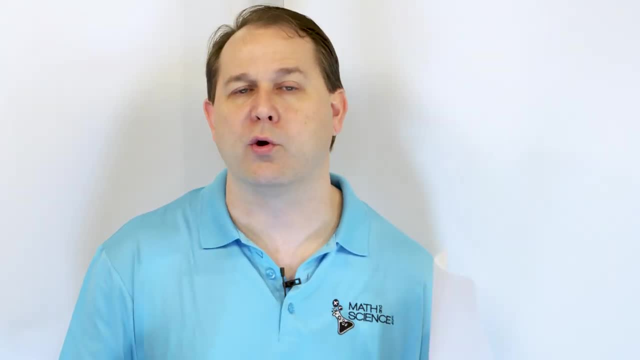 polynomials get higher and higher, like, let's say, a sixth order polynomial or a seventh order polynomial. there's not a good, clear way to just figure out the roots. I mean, now we can use computers to do it. But I'm not going to do that. I'm going to do it with a computer. I'm going to. 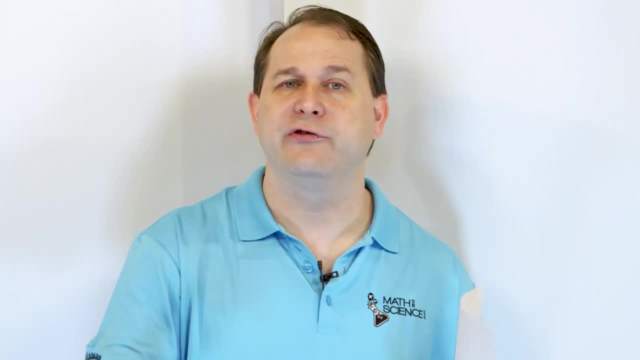 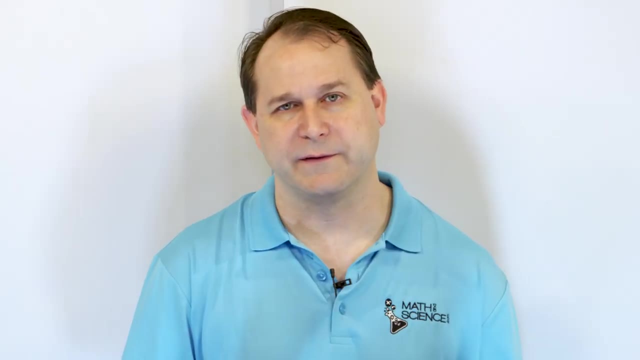 do what I'm talking about by hand. to actually find the exact solution to a tenth order polynomial is not something that we know how to do in algebra, But we do have this concept called Descartes' Rule of Sines, And it allows us to predict the possible number and the possible types of roots that a 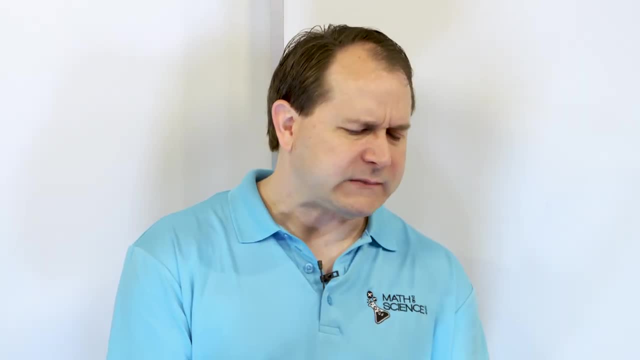 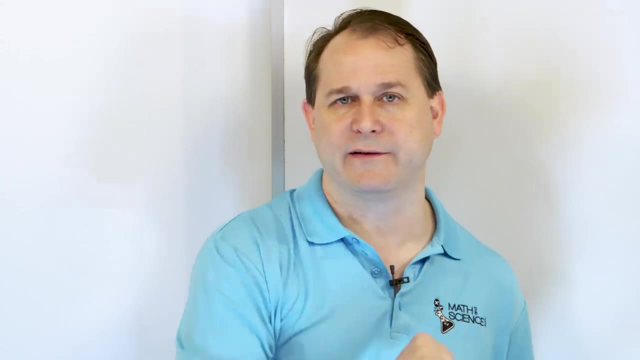 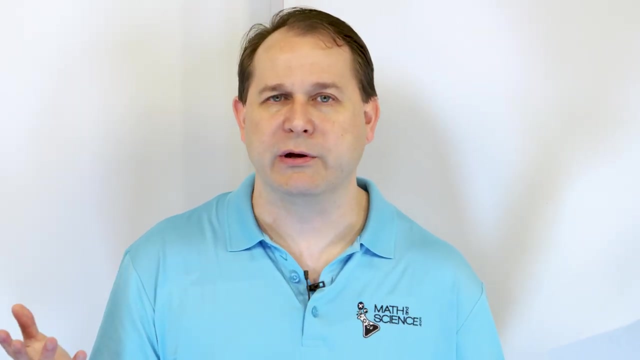 polynomial of any order can have. In other words, how many positive roots will the thing have? In other words, one, two, three, four. how many positive roots will it have? How many negative roots will the thing have? And then, because we know the total number of roots of any polynomial, 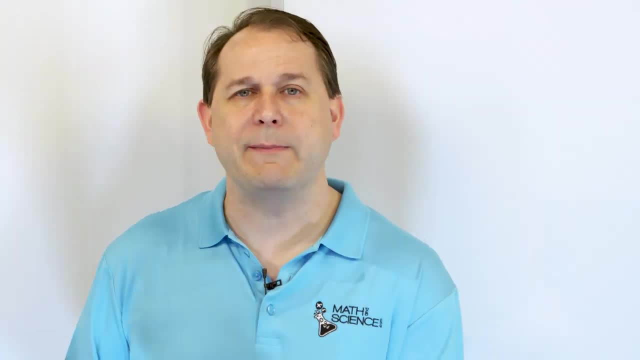 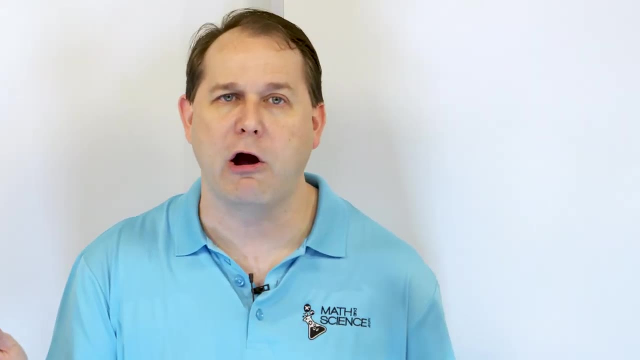 then we can oftentimes figure out how many complex roots. So we may not be able to actually find the actual value of the roots, But using Descartes' Rule of Sines we can figure out how many roots there are and the different types. So often the problem will say: here's a polynomial. 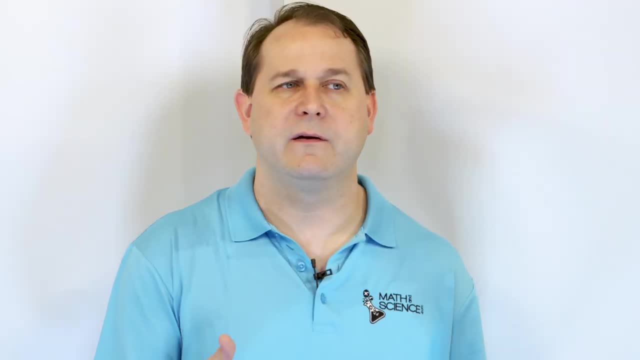 find the nature of the roots, And what they want you to tell them is they want you to tell them how many positive roots, how many negative roots, how many complex roots does the polynomial have, even if you can't find them, So we can figure out how many roots there are and how many types of roots. 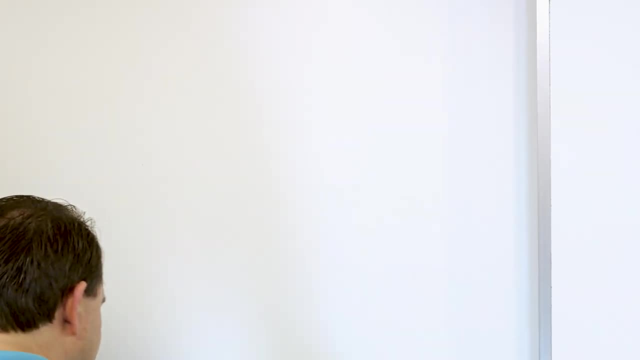 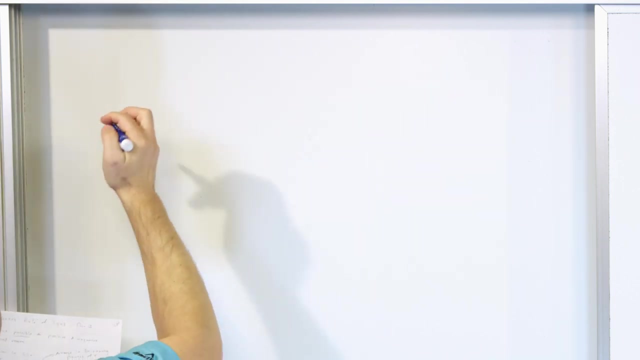 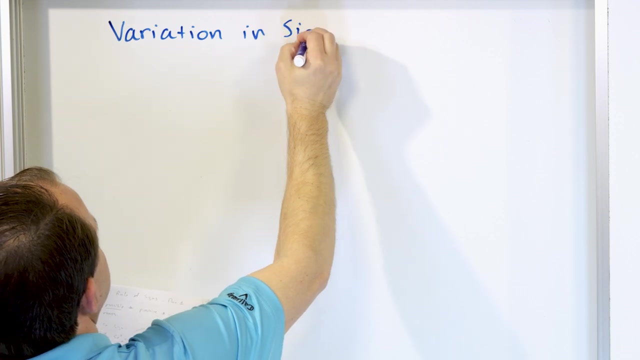 you can actually solve them. So, in order to do this, we have to learn about something called variation in sine, because it's basically what the Descartes' Rule of Sines is based on. So this thing is called variation in sine, And it's just much, much easier to explain it with an example. 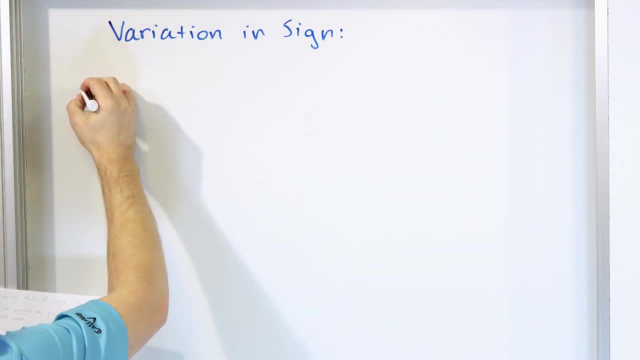 It's actually really, really simple. So let's take the first one. Let's say we have a sixth order polynomial that goes x to the sixth power minus two, x to the fourth power minus five, x to the second power plus three, x minus six. Now the first thing. 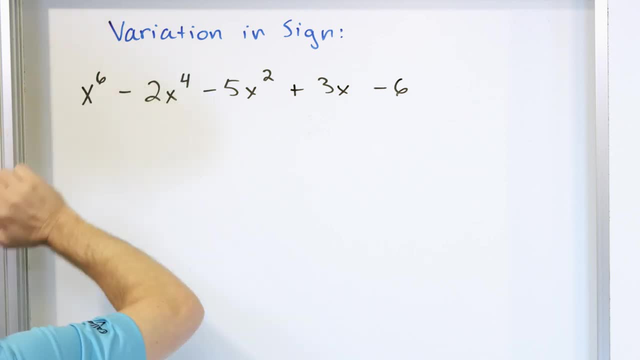 you need to do is you need to arrange the polynomial in order to figure out the variation in sine. You have to arrange the polynomial in decreasing degree of x, So six. there's no fifth power term, then four. there's no third power term, then two, then there's no. yeah. 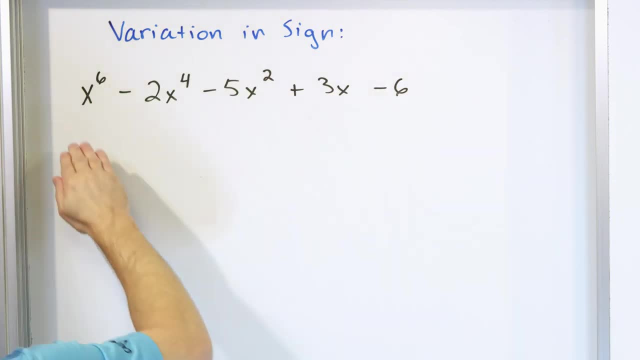 there is a one power term right here And then the zero power. the constant term is on the end, So you have to write it in in decreasing order And then you look for changes in sine. So you see how this first term is. 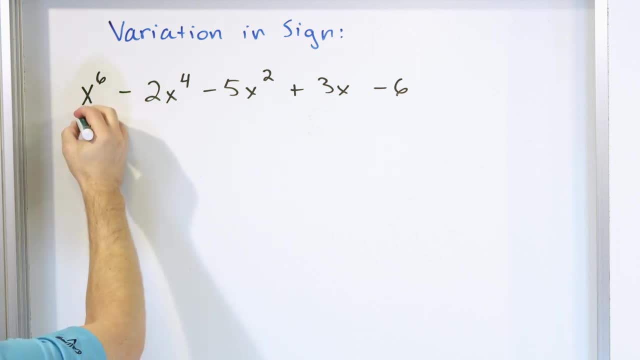 positive. There's an invisible positive here, but the next term is negative. So this means there is a one variation in sine, But when we go from the second term to the third term, see this one's negative but the next term is also negative. So this is not a variation in sine between those. 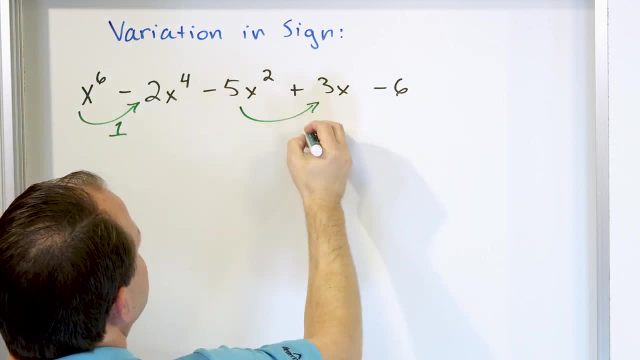 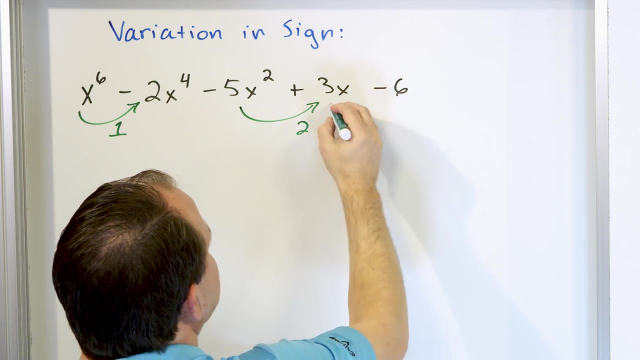 terms, But this one's negative and this one's positive. So this is number two. I'm numbering them. Number one, first: variation in sine. second, variation in sine. This one goes from positive to negative, So it's also a variation in sine. So there are actually. 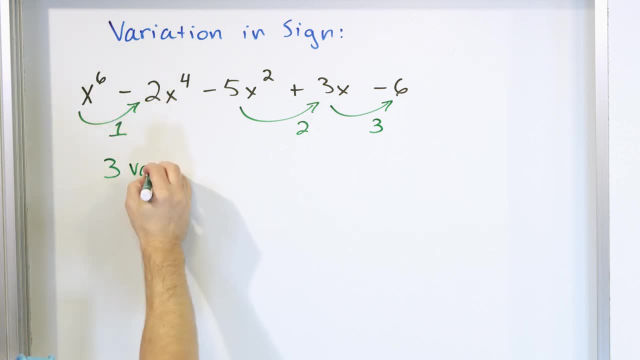 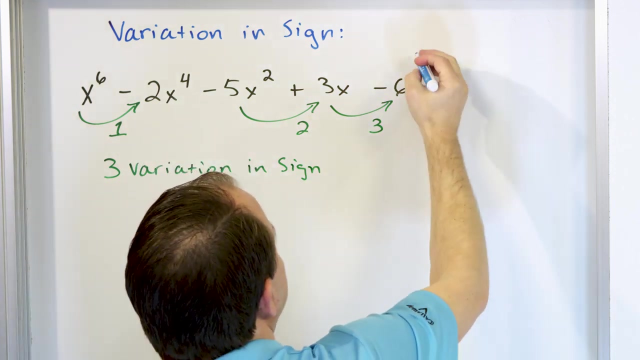 three variations in sine, in this polynomial, three variations of sine or in sine. And then one more thing I want to note. I'm not going to write it down for every problem, but you see how we didn't have a fifth order term, a fifth power term, We didn't have a third power term. So to figure out, 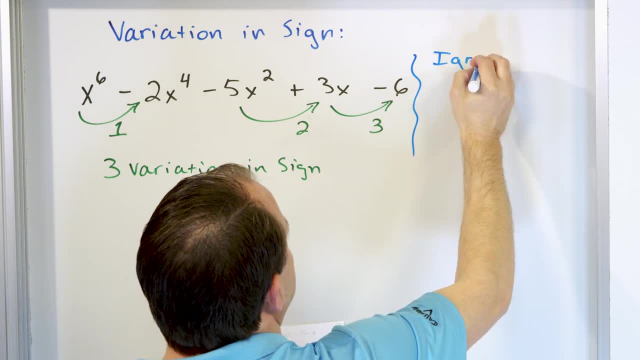 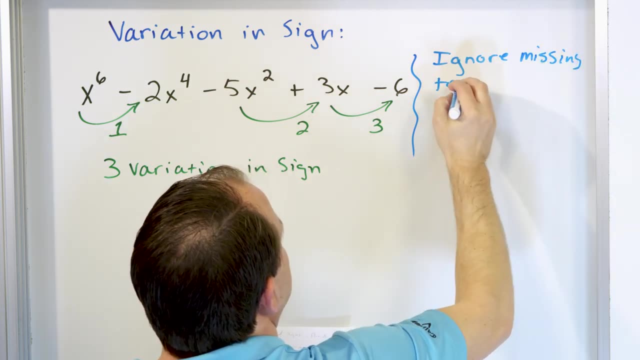 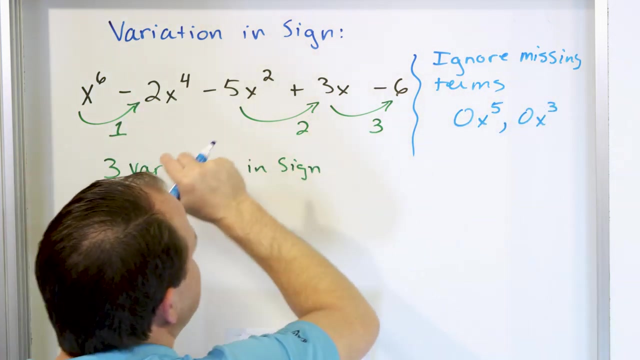 this variation in sine. you're going to ignore all of these missing terms, Like I'm just going to write it down. Missing terms, For instance: zero. there's a zero x to the fifth power in here, because it's missing. There's a zero x to the third power in here. that's missing. So we're ignoring those. 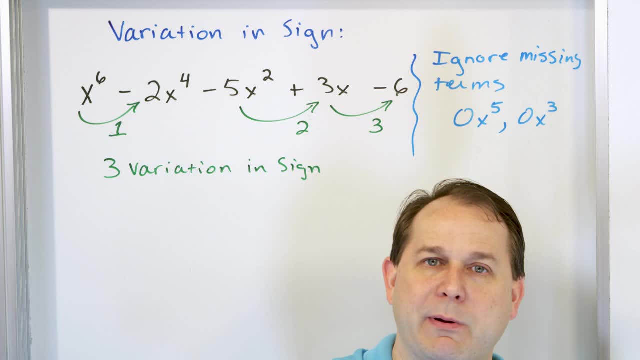 We're not, because zero really doesn't have a sine. Zero is neither positive nor negative, So we just ignore those. We look for the variation in sine. Now I haven't told you yet what Descartes rule of sine is, but you have to figure out how many variations in sine you have for a polynomial. 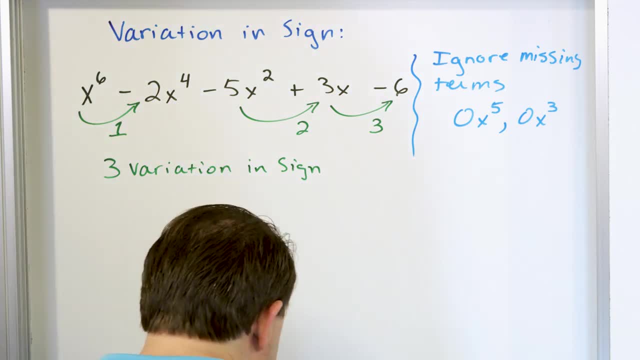 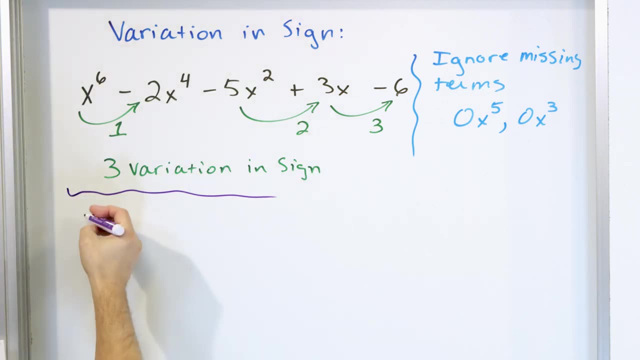 in order to use it. So that's why we're doing that first. All right, let's do one more little practice with variation in sine before I actually tell you what Descartes rule of sine really is. The next polynomial is: let's say we have a fifth order polynomial: x to the fifth plus x to the fourth, power minus 3x. 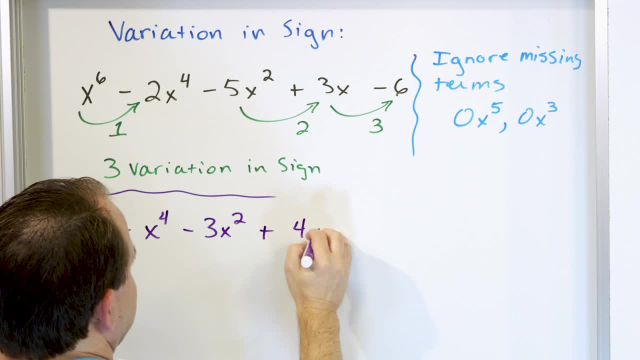 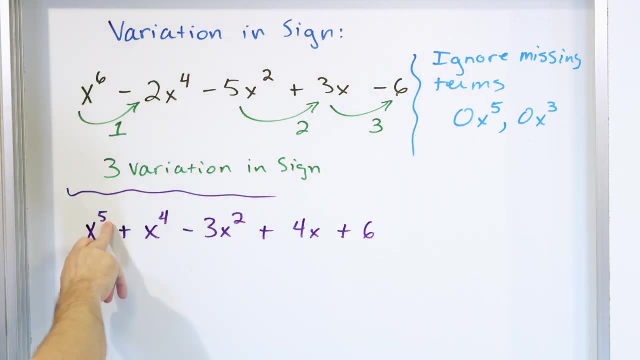 to the second power plus 4x plus 6.. So this is a fifth order. We know that this is a sixth order. This polynomial has six roots and this is a fifth order polynomial. It has five total roots, But we're now looking for the variation in sine. Positive, positive: there's no variation in sine. 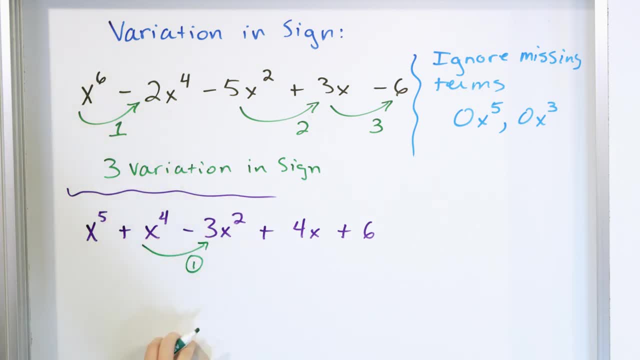 here: Positive, negative. there's a variation in sine right there: Negative to positive. there's a variation in sine right there: Positive to positive. there's no variation in sine here. So what I actually have here is two variations in sine. All right, so it's important now. 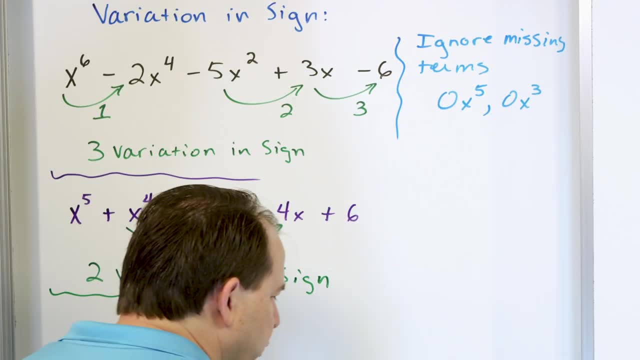 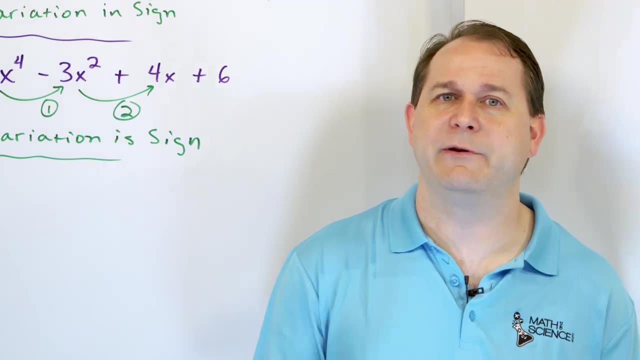 we're going to kind of put it all together here. We're going to write Descartes rule of sine down. it looks very complicated. When I write it all down, you're going to be like, whoa, this looks so complicated, It's not complicated. Trust me, just let me get through it. I have to. 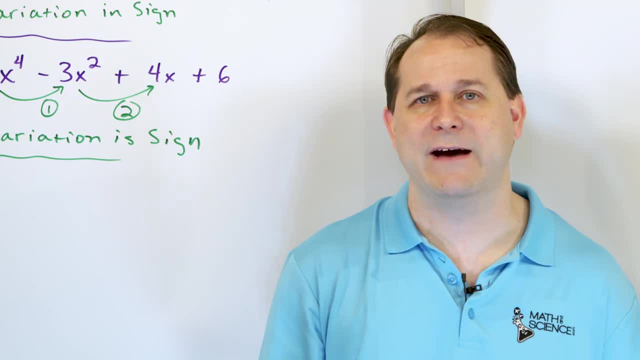 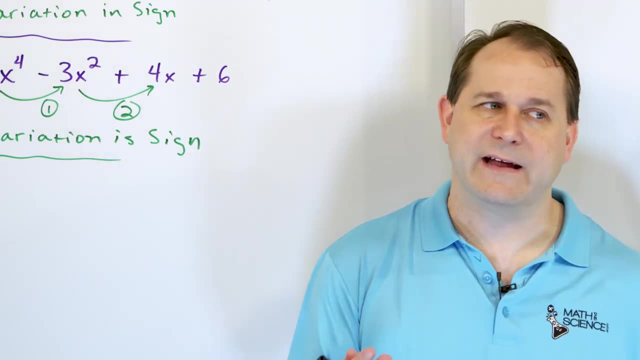 write a few things down, but it's actually one of the simplest theorems that we have in algebra. But the key to it is understanding how many variations in sine you have in the polynomial that you're given, because that's how the thing is written. That's how the theorem is written. 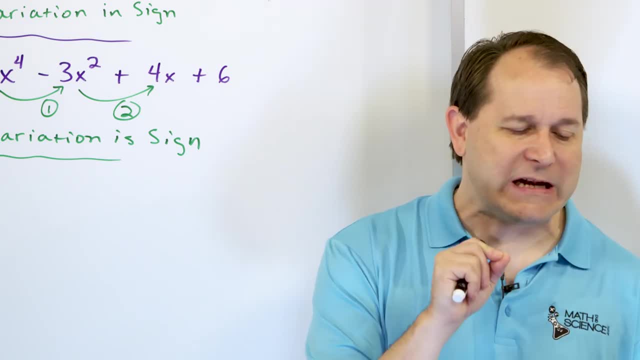 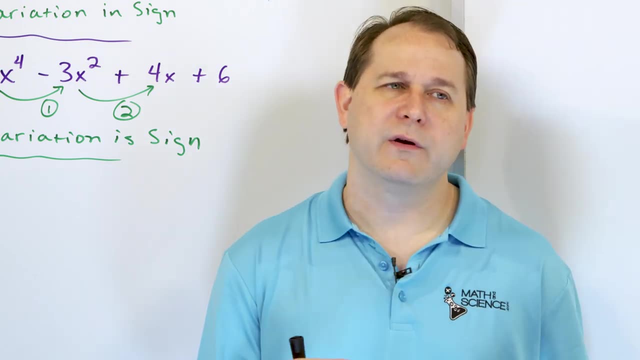 The most important thing I want to say before I write it down is it only tells us the number of possible positive roots and the number of possible negative roots. In other words, Descartes rule of sine doesn't give you a concrete answer. It's hard to describe without. 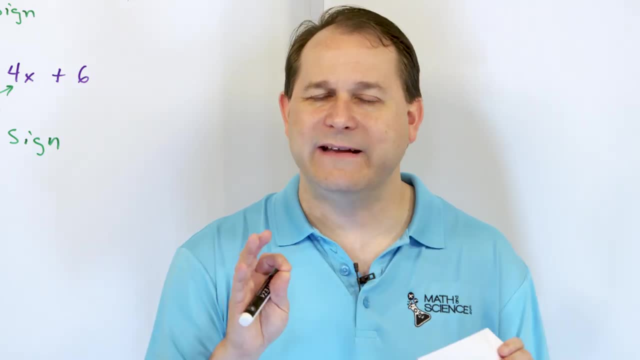 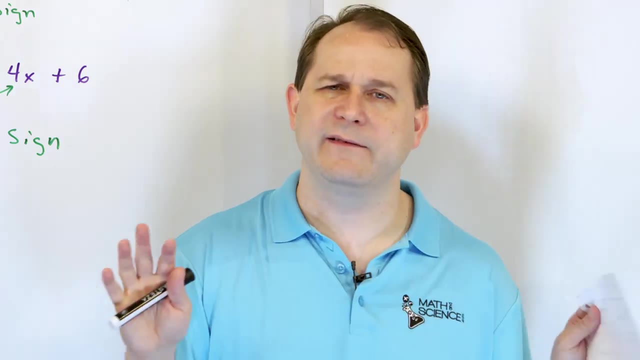 a problem and we're going to do a problem, so don't sweat it, we're going to get there. But it doesn't tell you, hey, you have five positive roots and two negative roots. It doesn't tell you, hey, we have one positive root and three negative roots. It doesn't tell you. 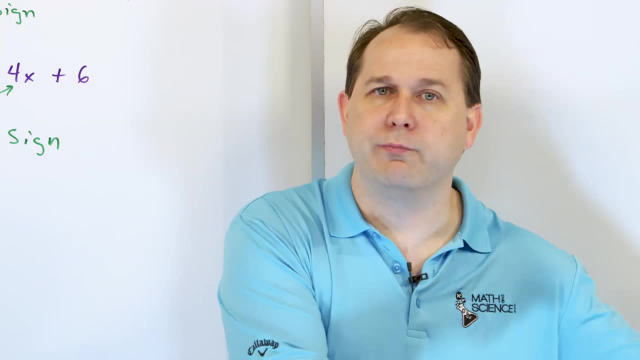 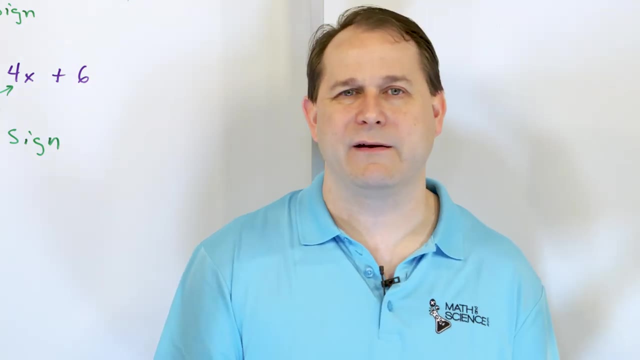 those things. It tells you you might have one or two positive roots and one or three negative roots. It gives you possibilities. It doesn't give you concrete things. So you might say, well, who cares about that? Trust me, in higher level you're going to get a lot of positive. 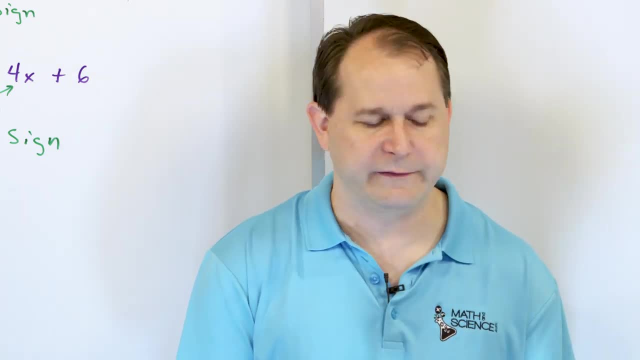 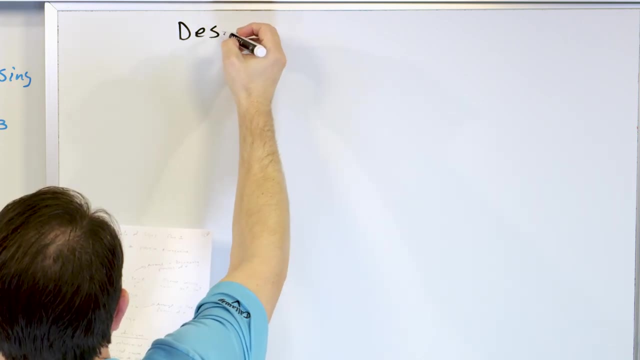 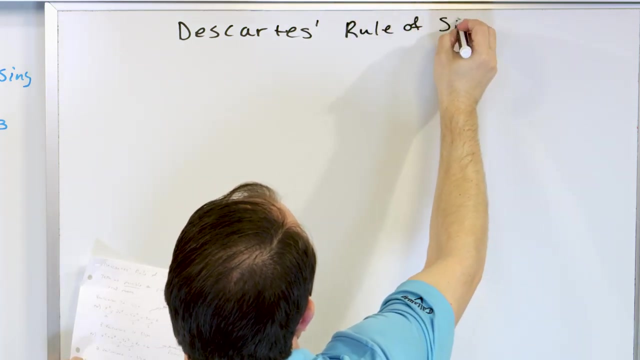 results. But in higher level math, if you're trying to solve a higher level polynomial, it has its uses. So let's go ahead and write it down And it's called, as we have said, Descartes. that's how you spell it: Descartes: rule of sines. All right, I'll be 100% honest. 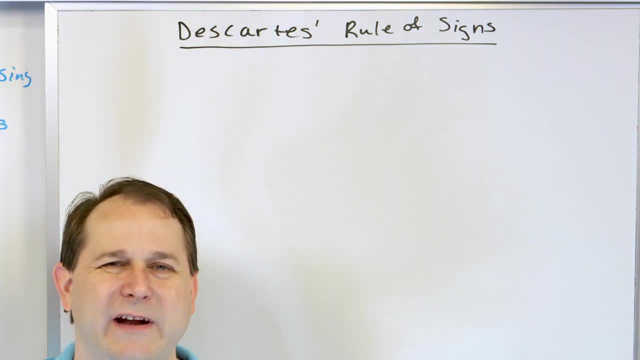 with you When you get into higher level math. you might use this a little bit. but for everyday use in algebra it's not something you use very much. But as far as the theory of algebra, the theory of roots, of polynomials, it's centrally critical to that, All right. So I'm going to kind of 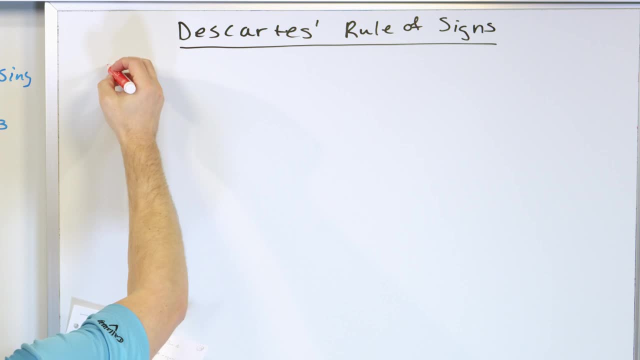 simplify this, So let's let. I'm going to do it in a shorthand way. In other words, you're going to see a much longer version of this in your book, So I'm going to say: let p of x be a polynomial. 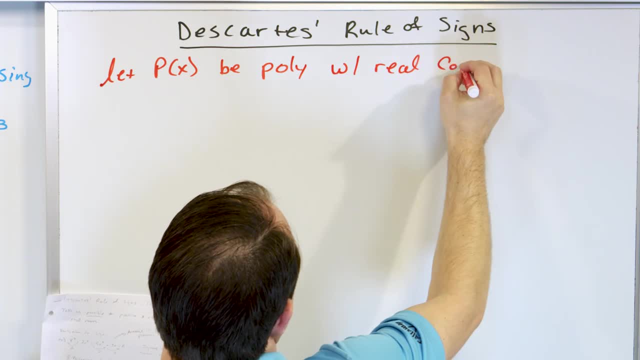 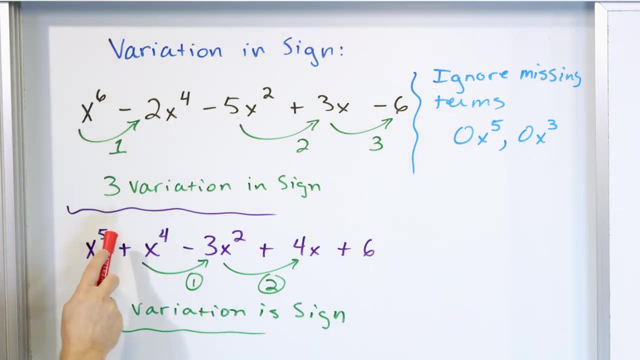 with real coefficient. That's pretty much every polynomial that we have, Every coefficient of this, all the terms in this polynomial, they're all real numbers. In other words, you don't see any imaginary numbers or complex numbers anywhere in here. All of the coefficients are just numbers. 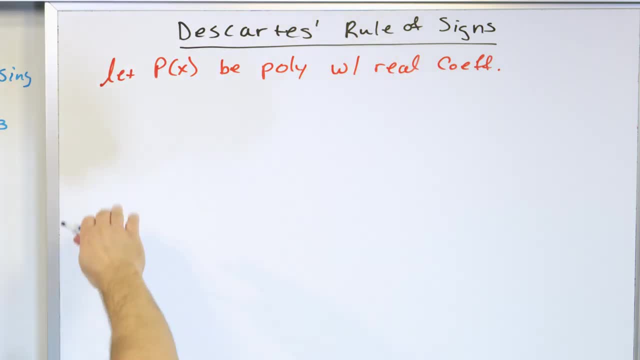 negative and positive numbers, All right. So let's let some polynomial be a p of x, have real coefficients, All right. So there's two parts to Descartes rule of sines, All right. The number of positive, oops, positive. I think I misspelled positive, Sorry, Positive. 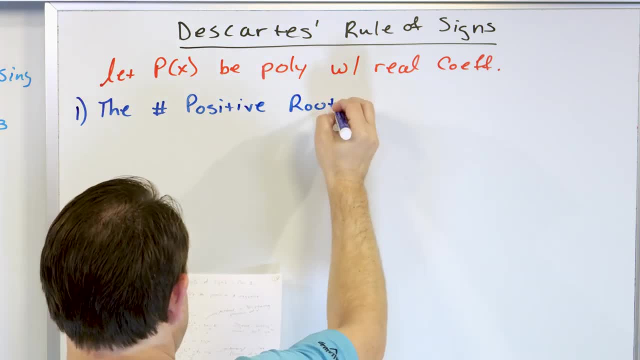 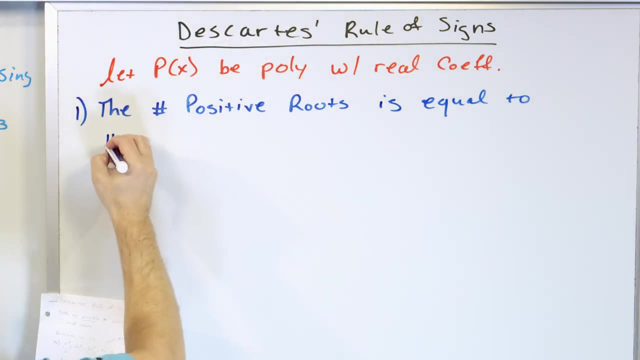 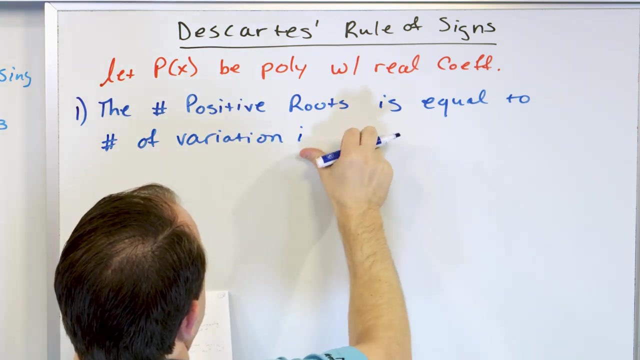 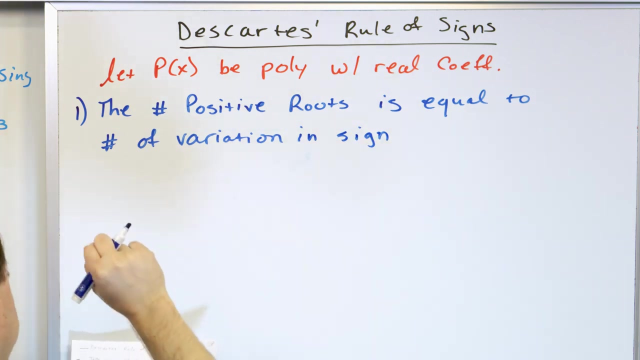 yeah, Number of positive roots is equal to the number of variation in sine. Now, this would be easy if it would just stop here, right? But it's not equal to the number of variation in sine. It's equal to the variation of the number of sine of the polynomial variation. 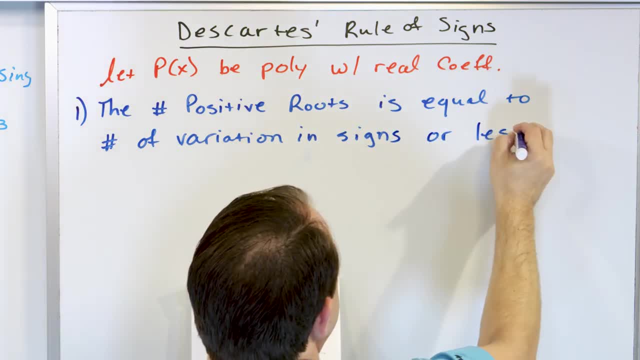 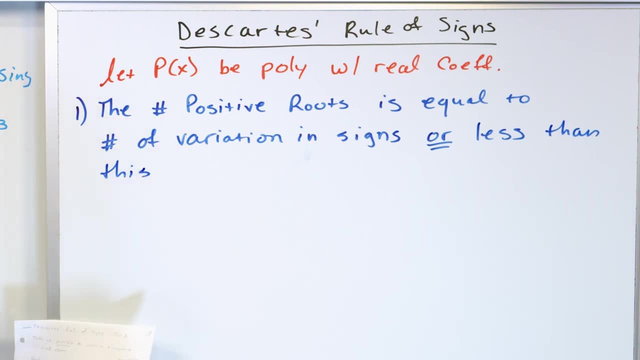 in sine to the polynomial, Or less- this is really important- or less than this by an even number, All right. So the bottom line is, if you want to know how many roots, how many positive roots, a polynomial has- when I say positive roots, I mean: 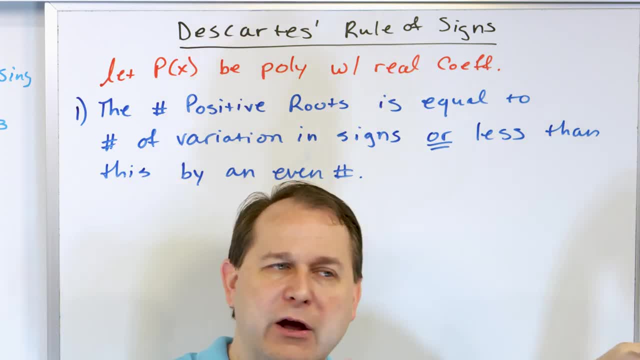 roots that are like one, three, five, four, two, anything on the positive side, positive numbers that are roots, then Descartes, rule of sine, tells you that, But it doesn't give you a concrete answer. It doesn't give you a concrete answer. It doesn't give you a concrete. 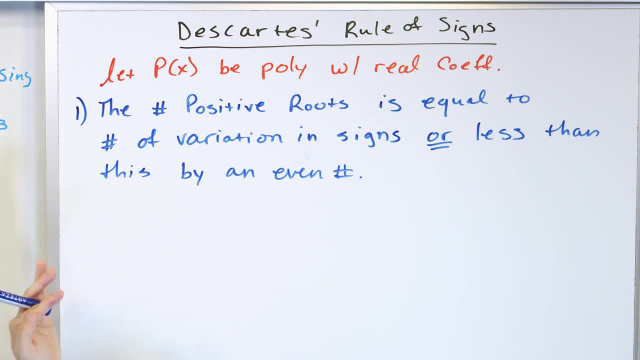 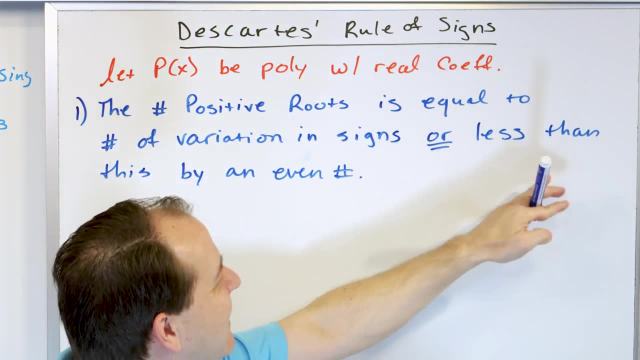 answer because if you find the number of the variation in sine there, it's telling you that the number of positive roots is equal to the however many variation in sine you found, or it can actually be less than that number, but not just less than it, it can be less than that. 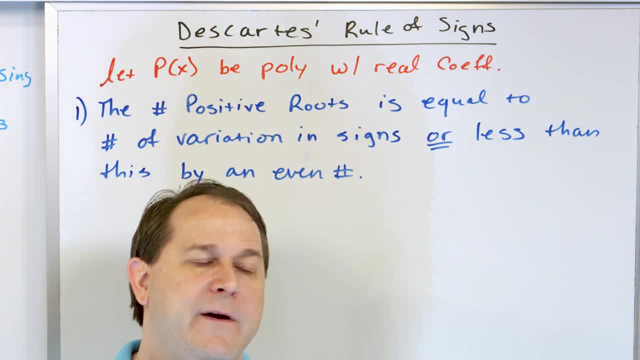 number by an even number. So, for instance, if you have five variations in sine, then the number of positive roots can be five or three, because that would be two, that would be an even number less, So it could be three positive roots. Or you can't find the number of positive roots in the number of 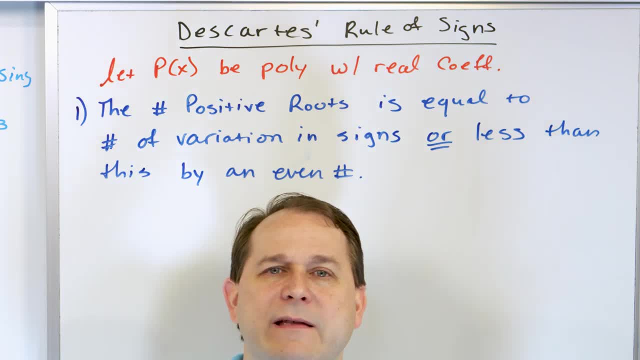 one positive root, You see. So the variation in sign tells you the maximum number of positive roots. but you could have less than that, but not just less than it. It can be less than that number by an even number, meaning you have to count by twos down. Basically, that's what even numbers. 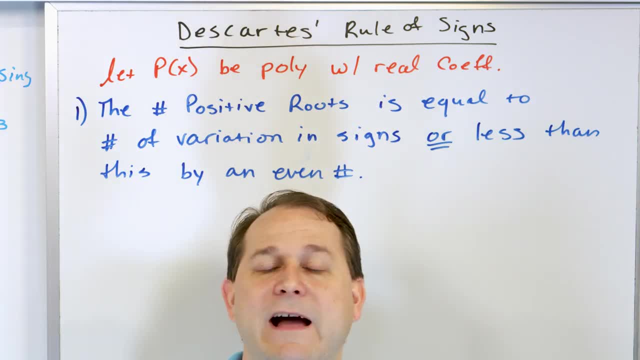 are when you count by twos. So if you had five variation in sign, you'd have five positive roots or three positive roots or one positive roots. Descartes' rule of sign doesn't tell you how many you have, It tells you the possibilities. But you know for sure that if you had a polynomial with 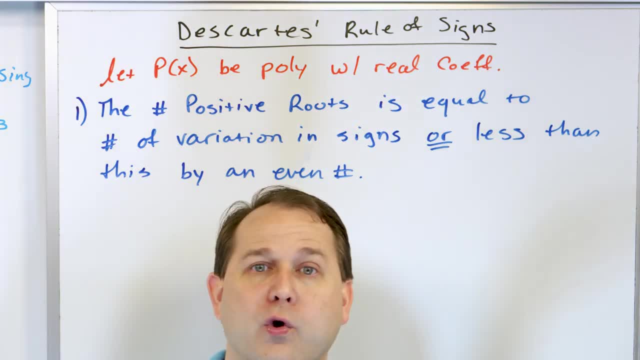 five variation in sign. you will definitely not have four positive roots, because you can't. If you had five variation in sign, then it has to be that or less by an even number. It can't be four. You have to count by twos down. You can't have, for instance, zero positive real roots. 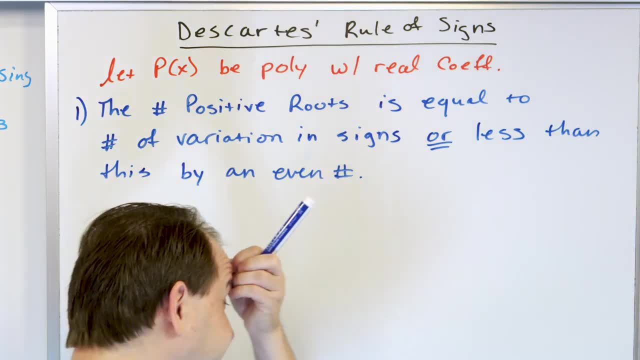 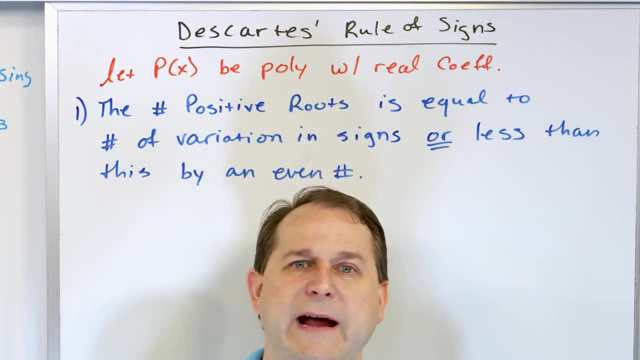 because it's not an even number, less as well. Now there's a part two to this. You might say: well, this tells me how many positive roots I have, but what about the negative roots? What about negative one being a root? What about negative seven? What about negative eight? 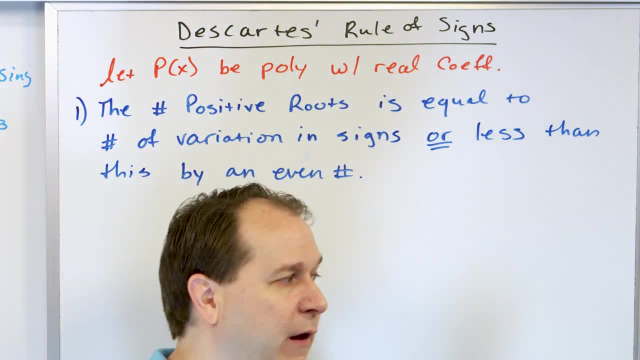 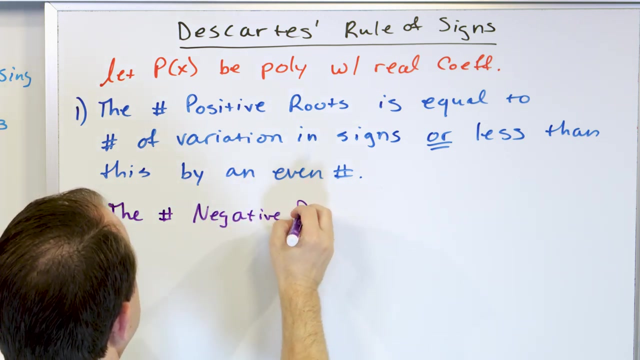 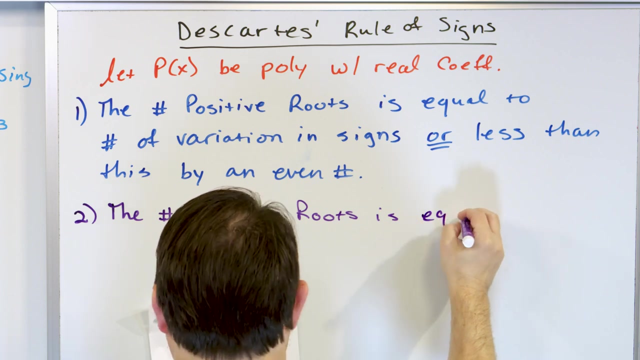 What about negative 17 being a root? What about negative one half being a root? How many of those roots do we have? So it's very similar to this, but you know, very similar. Let me just get it on the board: The number of negative roots is equal to the number of variation. 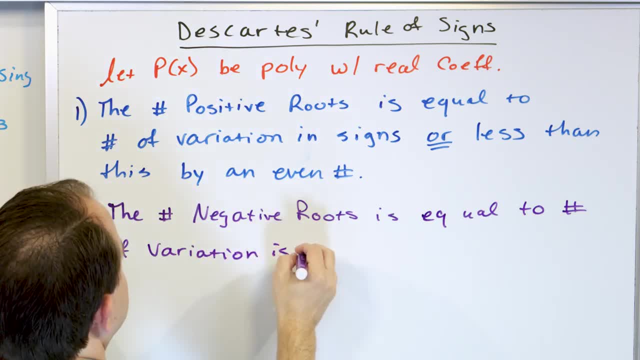 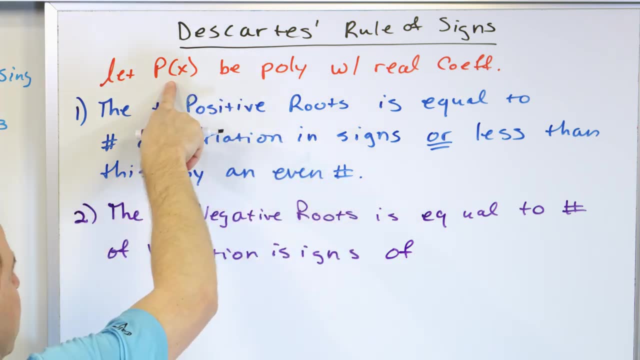 in signs of- and this is critically important- not the variation in sign of the polynomial you started with, but the variation in signs of the polynomial replaced with negative x. You see, replaced with negative x. I'll show you how to do that in a second And the same sort of thing at. 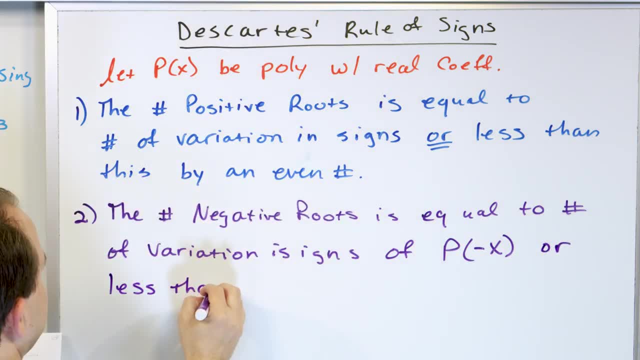 the end, Or less than this by an even number. Now it kind of makes sense that you have some positive roots, but it has something to do with negative x here, because you're looking for negative roots. So what you have is you have some polynomial, and we know how to figure out how many. 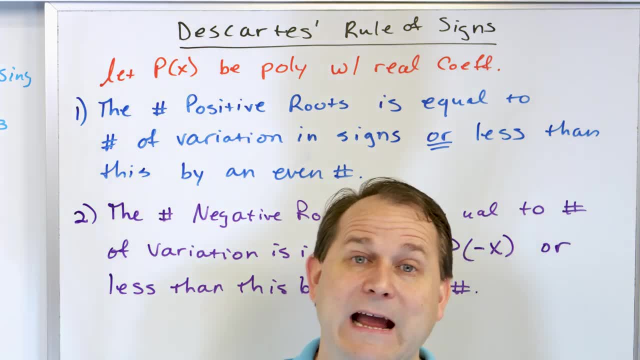 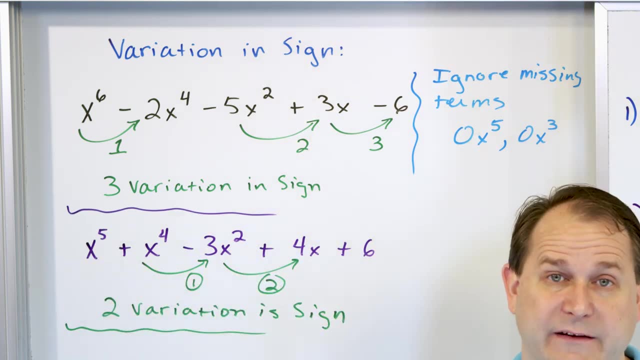 positive roots are possible, right. How do we figure out how many negative roots are possible? You take your polynomial, for instance. one of these here: Everywhere where you put an x here, you stick a negative x in its place. That's what this p of negative x means, You know. 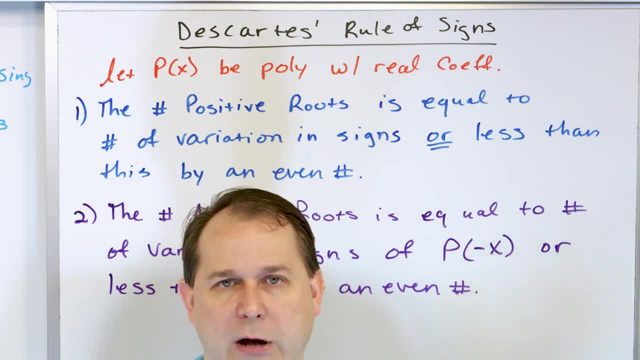 if you have p of one, then you put the number one into the polynomial. If you have a p of five, you put five everywhere where you see x in the polynomial. If you have p of 17,, you calculate by putting a 17 everywhere where you see x in the polynomial. If you have a p of 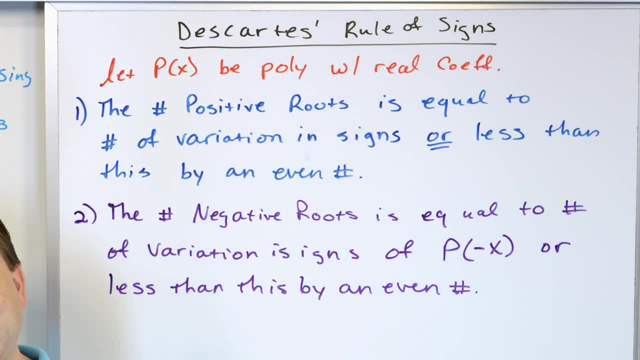 negative x, then everywhere where you see an x, you just stick a negative x in there. That's going to slightly change the polynomial, because you put a negative x in there, right, And you find the variation in sign of that version And then, however many variation of sign you have, is the. 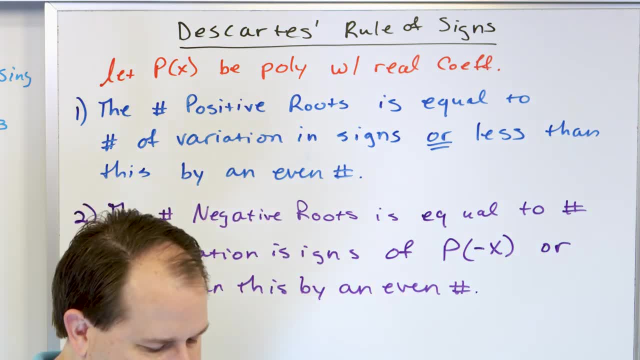 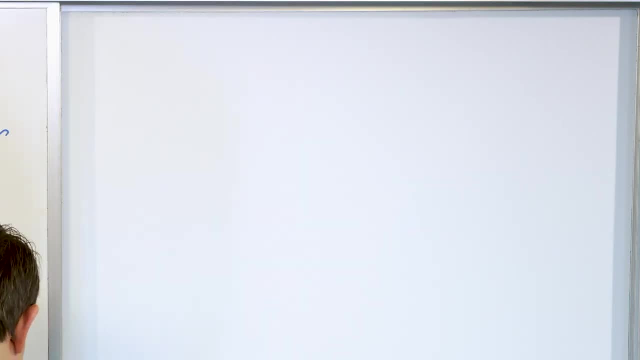 number of negative roots, or it can be less than that by an even number, Sounds really complicated because there's a lot of words on the board, but it's actually really easy. So let's go and do the fully, the full problem, So the way that this problem might go, it would say, list the nature. 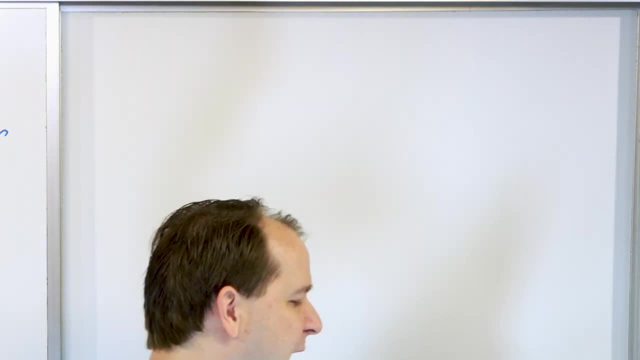 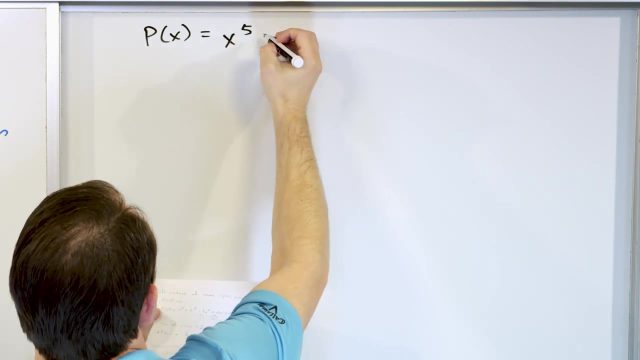 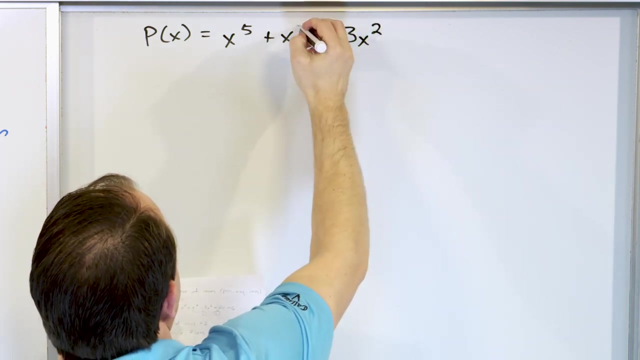 of the roots- positive, negative or imaginary roots- of the following polynomial. The polynomial is: p of x is x to the fifth plus x to the fourth, minus three x squared. Sorry, this is a fourth right here. Three x squared. Then we have four x. 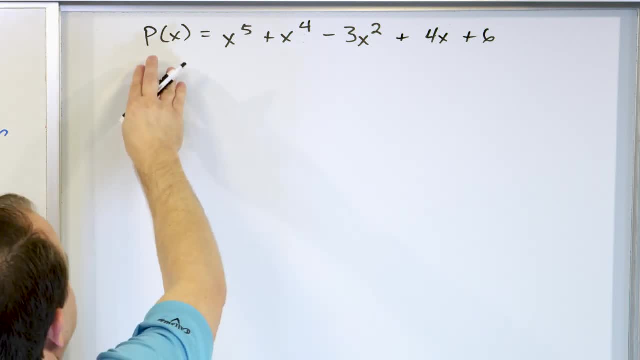 Then we have plus six, right. So we're trying to find the roots. And you know that roots mean that you take p of x and you set it equal to zero. So we want to find how many and what are the locations of those roots. So we look at the variation in sign to figure out how many positive. 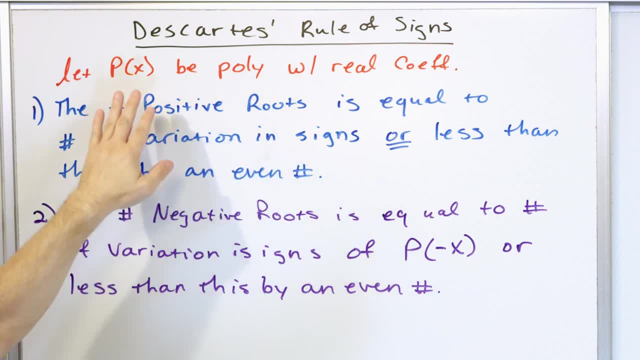 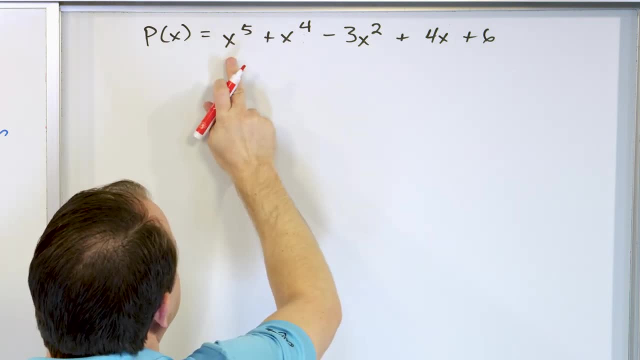 roots we could possibly have. We have to figure out the variation in sign of this polynomial that we're given. So this polynomial has a positive term. positive term And notice, first of all we wrote it in descending order of x, So that has to be done. So there's no variation in sign. 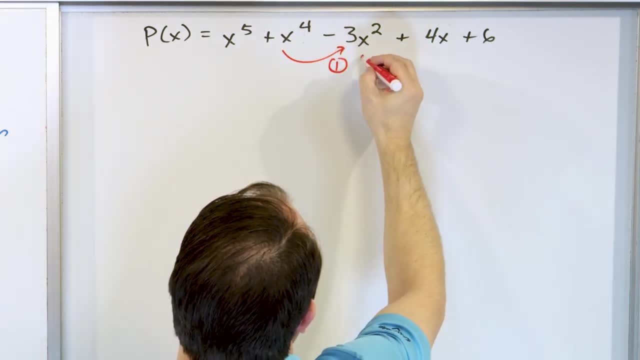 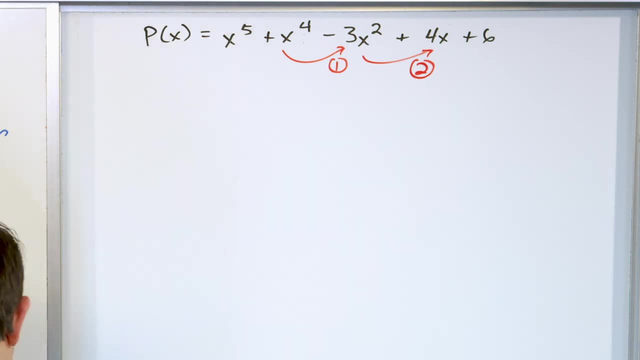 there. but there is a variation of sign. Then we have negative to positive Here. we have a variation in sign right here And positive to positive there. So what we have for the basic polynomial p of x is we have two variations. 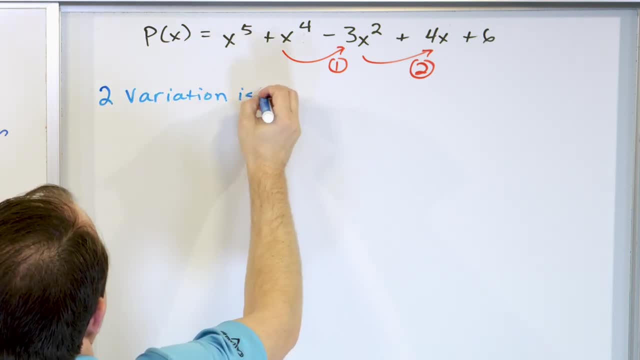 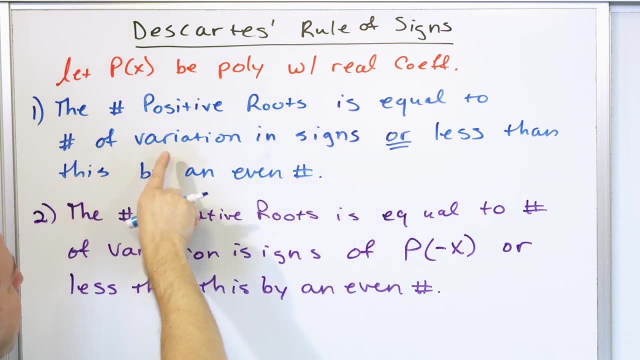 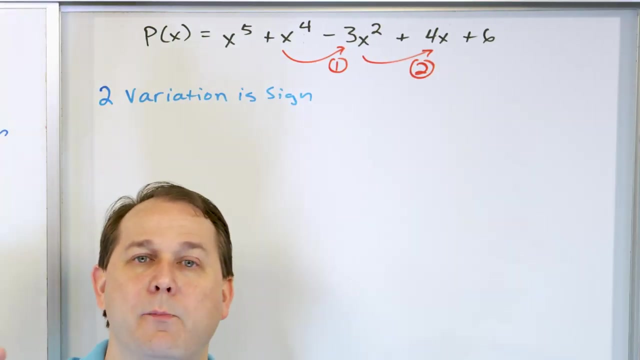 in sign, right. So what does that mean? It says the number of positive roots is equal to the number of variation in signs, or less than that number by an even number, which is a fancy way of saying you count by twos downward. That's all it's saying. So, since we have two variations in 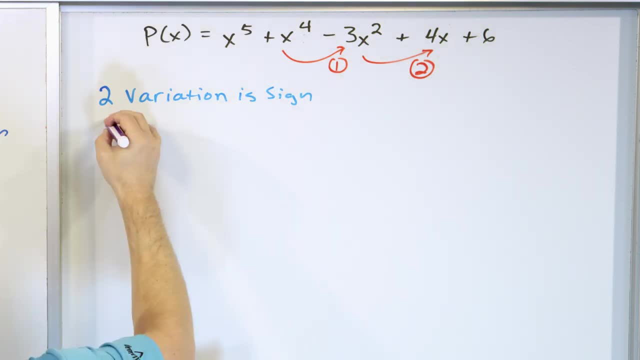 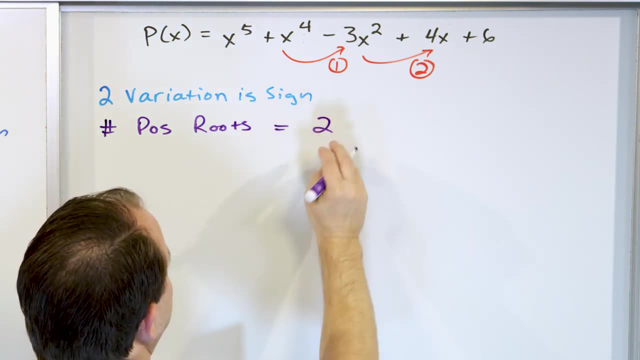 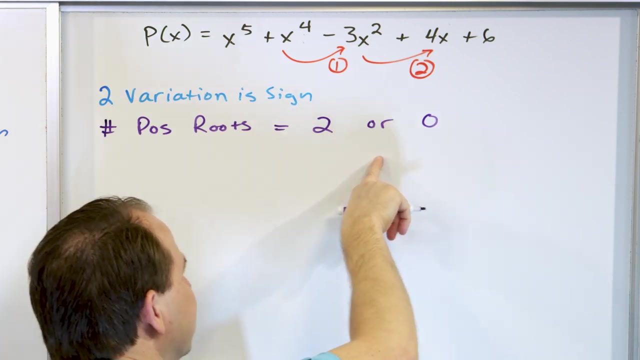 sign. what this thing is really telling us is for the number of positive roots. that's what the POS means. It means positive. It can equal two positive roots or zero positive roots, because this is less than by an even number. See, you start with two and you count down by two. You can't go down below zero anymore. 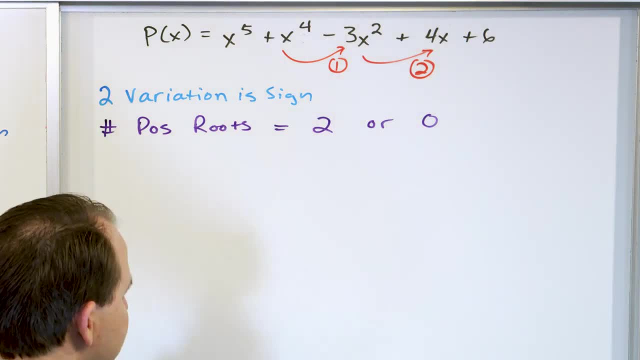 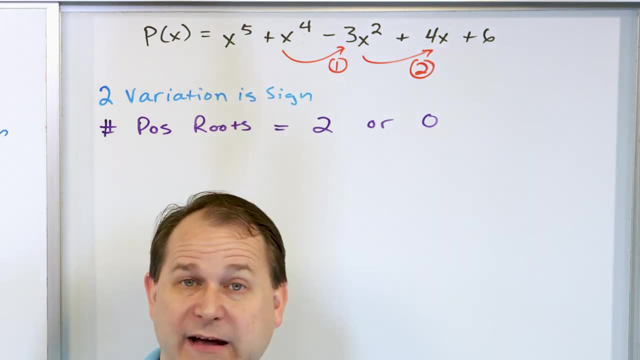 You can't have negative number of roots, So you basically stop there. So we know, we do not know, We don't know what the roots of this fifth order polynomial is, but we know that there's got to be five total roots because across real or imaginary roots, we have to have that. 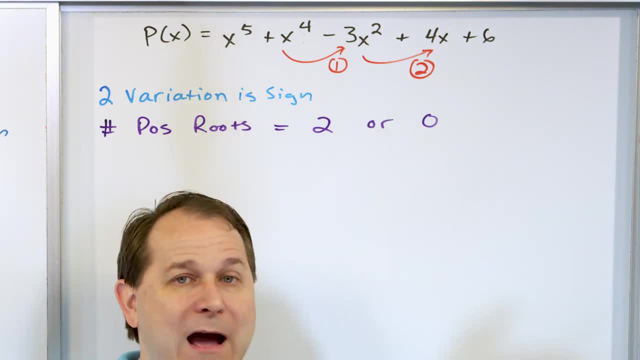 amount. We learned that a long time ago. right Now, we know that there could be two positive roots or there might be zero positive roots. We don't have any idea which We don't know. Descartes rule of sign doesn't tell us, but we know that we can't have one. We cannot. 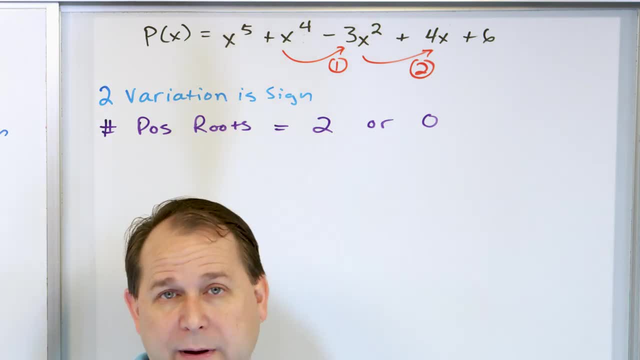 have one positive root. We cannot have three positive roots. We cannot have four positive roots. We cannot have five positive roots. We can only have two or zero. That's it. that's the only two possibilities. So it eliminates a lot of possibilities. 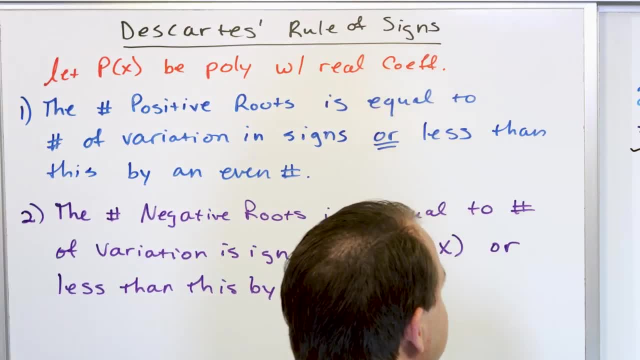 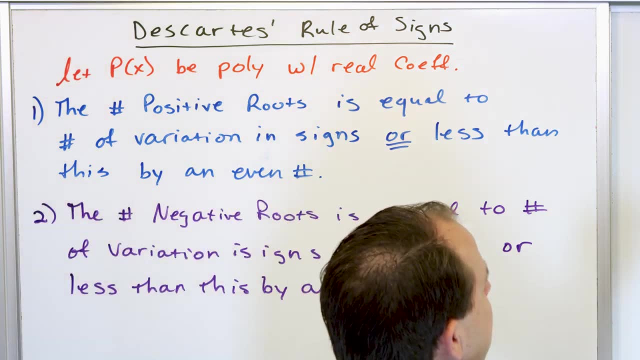 All right, so that's for the number of positive roots. Now for the number of negative roots. it says we have to do the variation and sign on a modified version of the polynomial. So what we do is we say: well, let me take this polynomial. 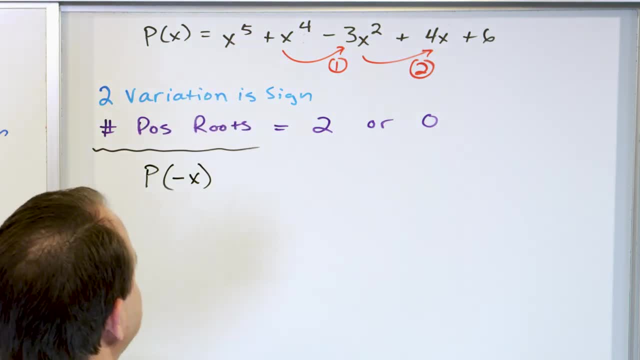 and I'm gonna stick a negative x everywhere I see an x. but you have to be careful, because you're raising everything to an exponent. you have to do it like this Negative x. you have to raise the whole thing to the fifth power. 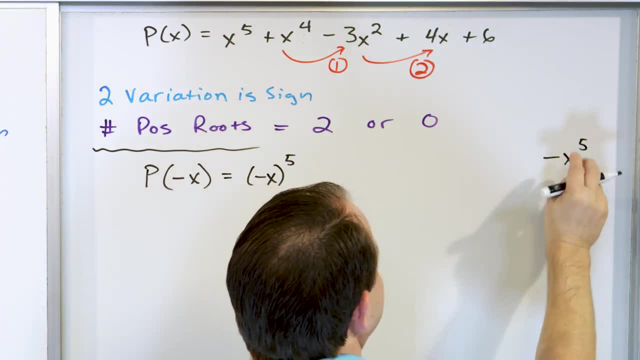 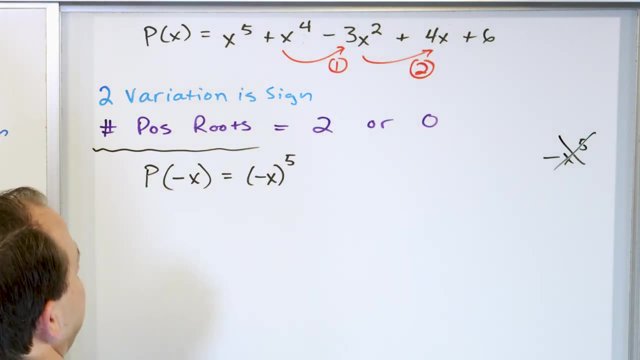 You don't wanna put like negative x to the fifth. that's different. You wanna take the whole thing because you're sticking it in to there. So you don't wanna do that. You wanna put it in and raise the whole thing, And we'll calculate the answer to this in the next step. 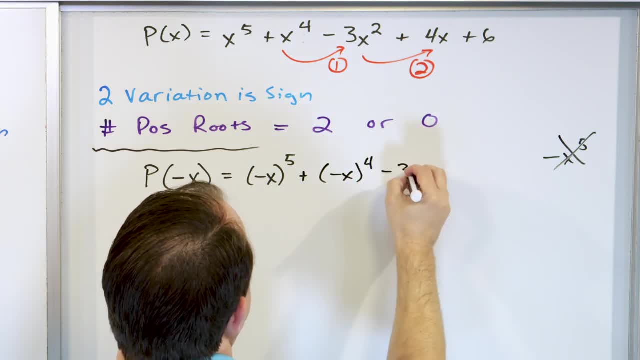 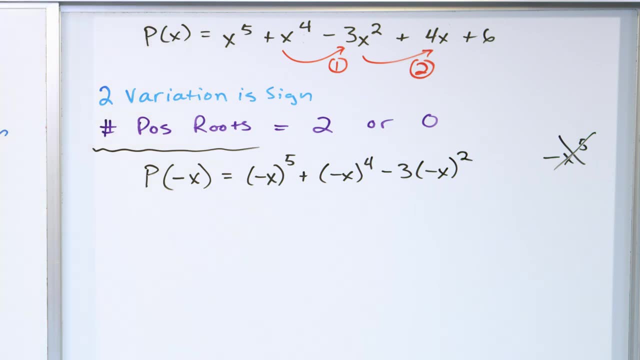 Then we have negative x raised to the fourth, Then we have negative three negative x raised to the second power, And you know what? let me go ahead and just take a look at this. Let me take a second and get this out of the way. 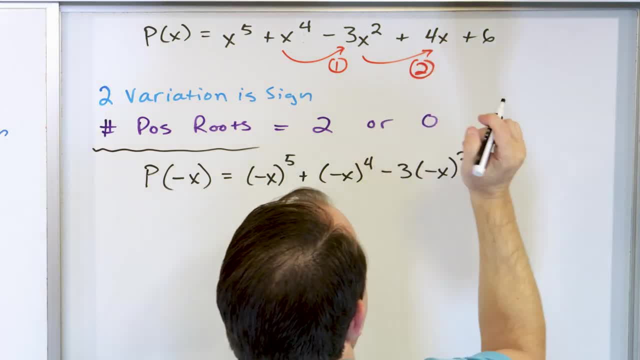 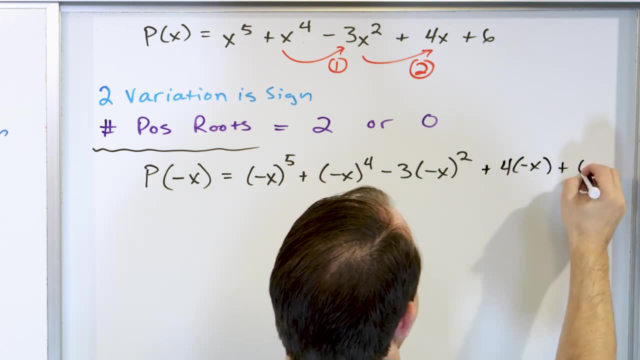 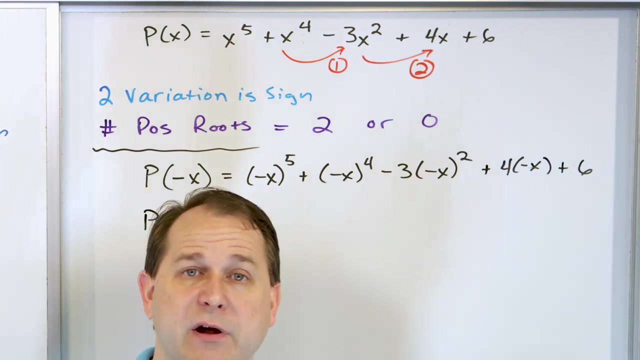 We don't wanna do that, We've decided we don't wanna do that. Then we have over here plus four negative x, And then we have plus six. So now what we have to do is calculate kind of the new version. Now you know whenever you raise negative numbers. 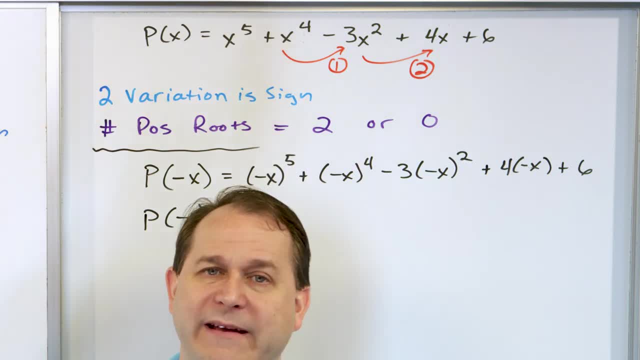 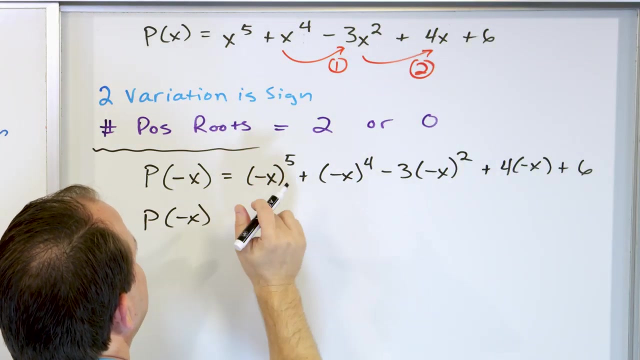 to an even power, then the signs go basically make it positive. When you raise a negative one or negative numbers or whatever, to odd powers, then the sign becomes negative because negative one times negative one and odd number of times makes it negative. So here we have this negative term raised five times. 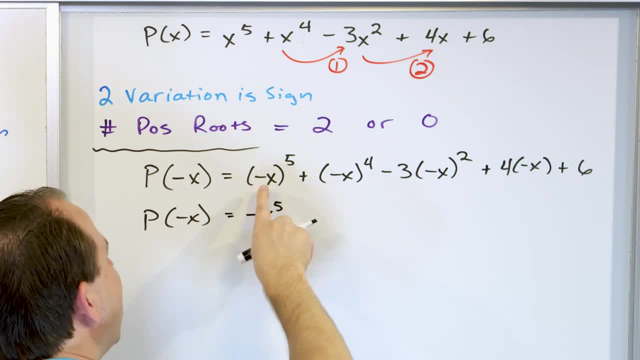 So what we're gonna have is a negative x to the fifth. So it worked out this way, because the negative one was multiplied by itself five times, which makes a negative in front. The x was multiplied by itself five times makes x to the fifth. 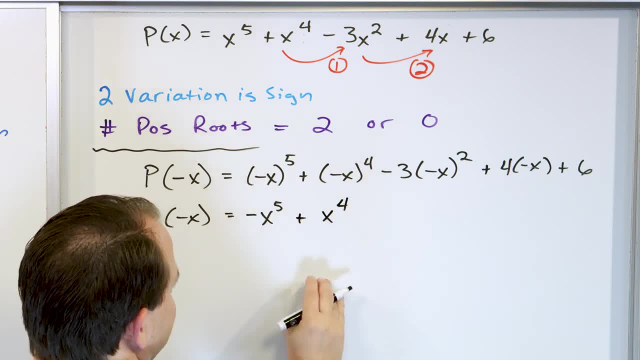 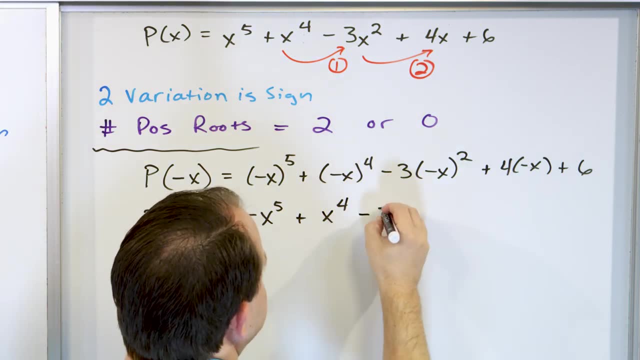 But here this negative basically goes away. We have a positive x to the fourth because the negative one was multiplied one, two, three, four times. That kills it and makes it positive. Here we have a negative three, But this negative x squared makes it a positive x squared. 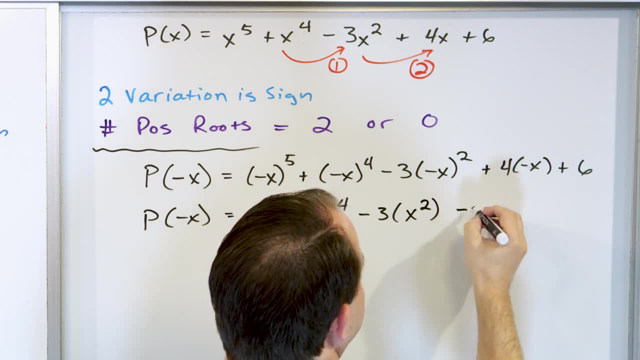 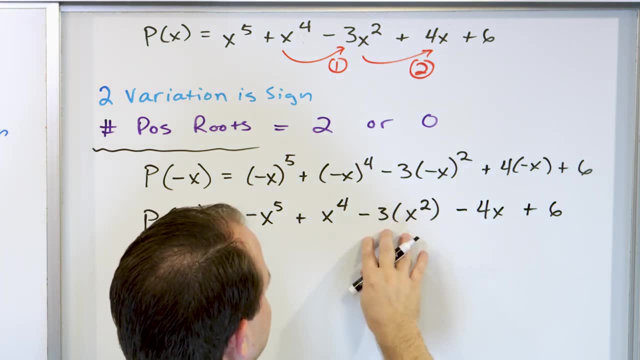 Right, we'll do the signs later over here. Then we have four times negative. x means negative four x, And then we have positive six. So really I put the parentheses around here, but you know you don't really need them. 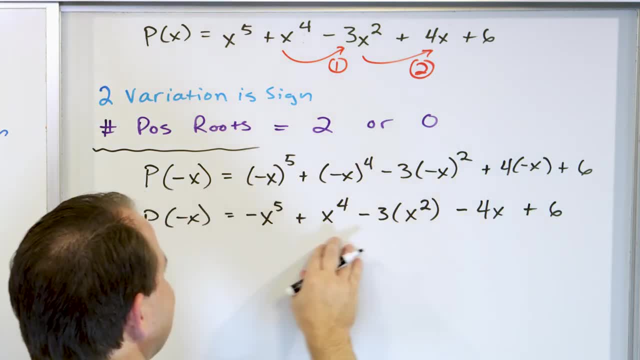 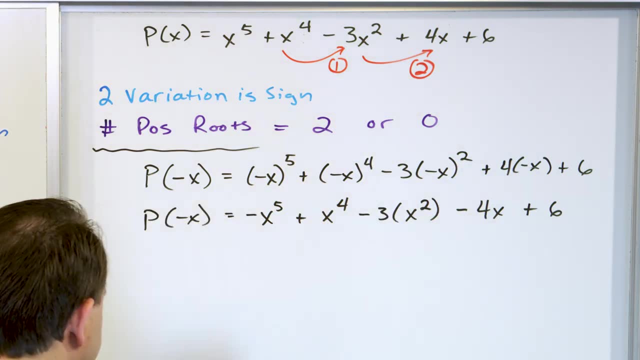 So I don't need to rewrite the thing again. I just wanna make sure you understand how we're getting the signs correct everywhere, And it's because of the way we're raising the exponent of the negative powers here. All right, so the next thing we're gonna do: 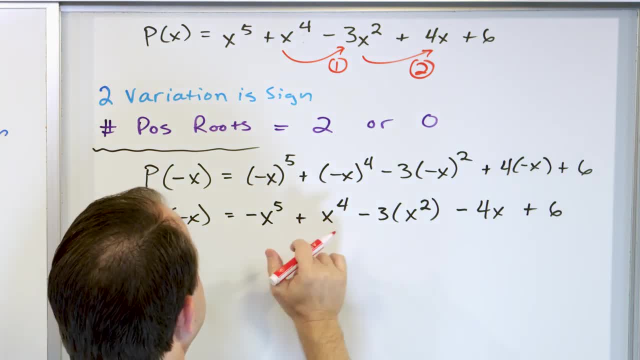 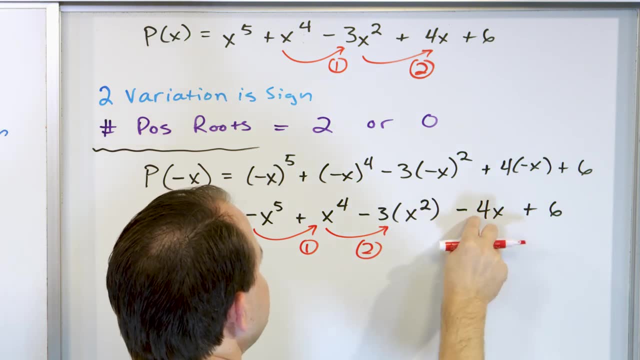 let me catch up to myself and make sure I've done everything correct. So this is a variation of sign going from negative to positive. This is a variation of sign going from positive to negative. This is no variation in sign, but this one is a variation in sign. 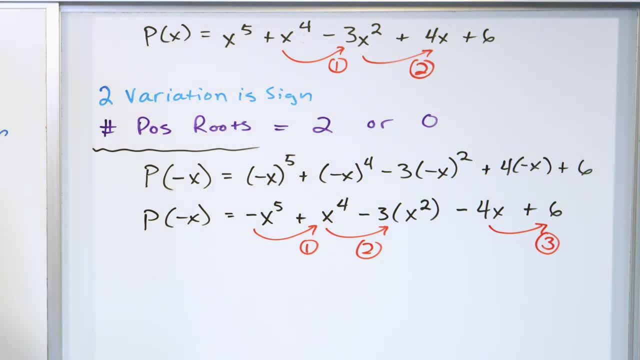 So there's your third variation in sign. So what this means is kind of mirroring what we did before. we have three variations in sign right, And so then from that we can figure out the number of negative roots. It has to equal one, two, three. 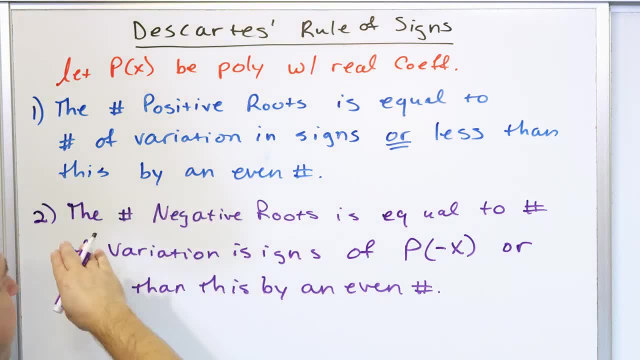 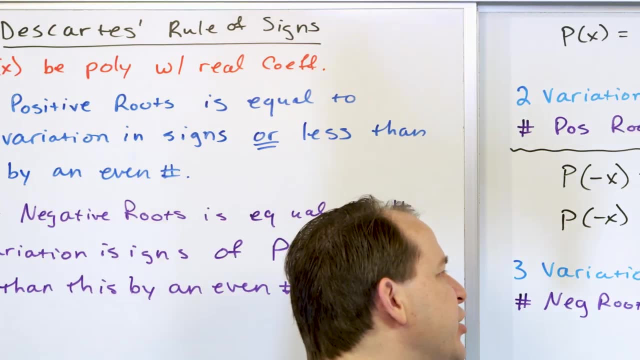 It has to be three, but according to the theorem, the number of negative roots is equal to the number of variation in signs of this modified polynomial, or less than that by an even number, which means you count down by twos. So it can be three or one. 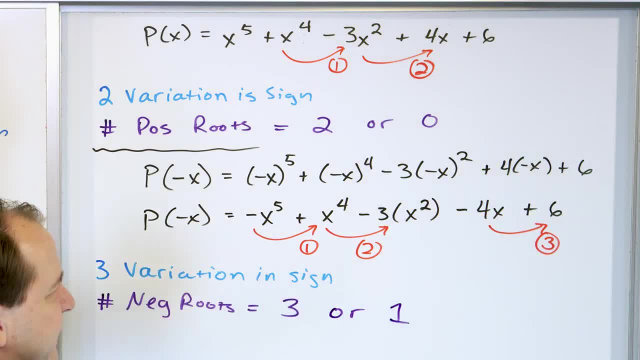 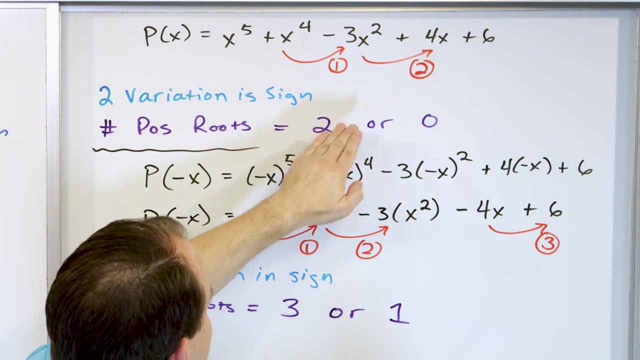 It can't be less than that, because you can't subtract two and still have a positive number or zero. So you see, what you have learned here is that you know that the number of positive roots of this parent's polynomial can be two or zero. 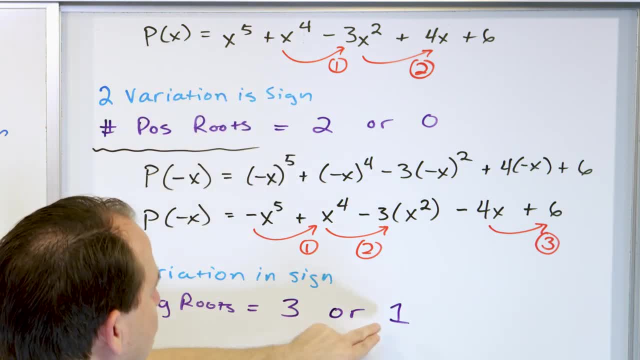 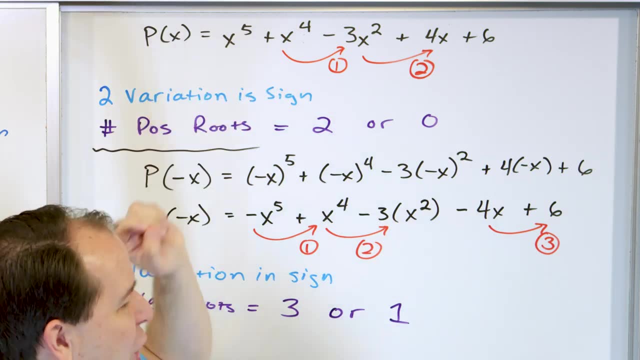 The number of negative roots can be two or zero. The number of positive roots of this parent polynomial can be three or one. But you see, you have a lot of possibilities, right? Because you know that you have five total roots- total. 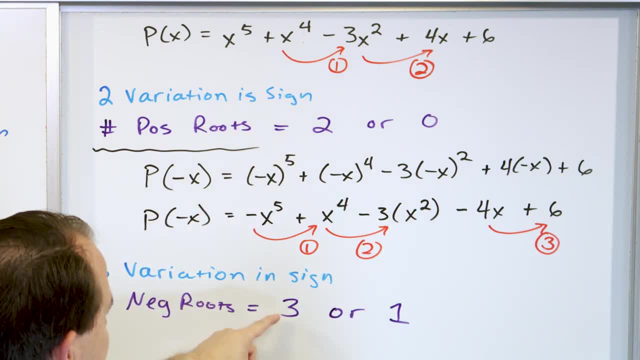 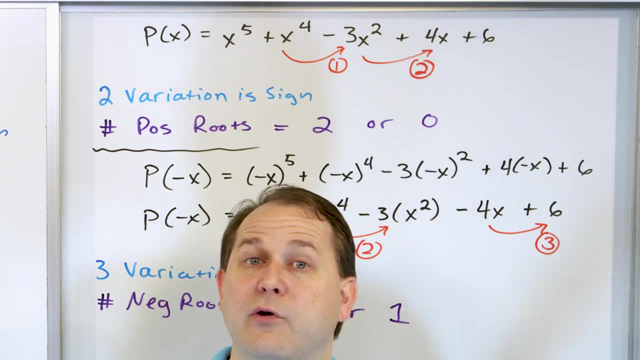 So do you have two positive and three negative, which would be five, or do you have some other combination of them? Because it doesn't tell you how many negative and how many positive exactly. it just gives you options. So we know, for instance, we cannot have two negative roots. 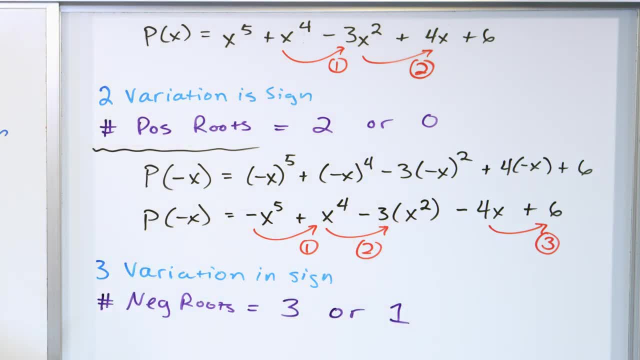 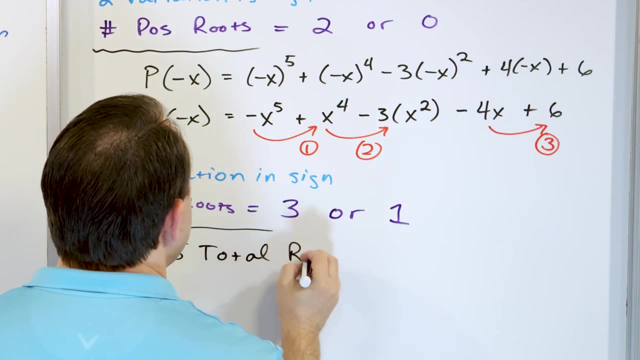 We cannot have four negative roots, for instance. So what we can do to do this is to write a table, And we know that there's five total roots of this polynomial. But don't forget that, for a polynomial in general, you can have positive roots, you can have negative roots. 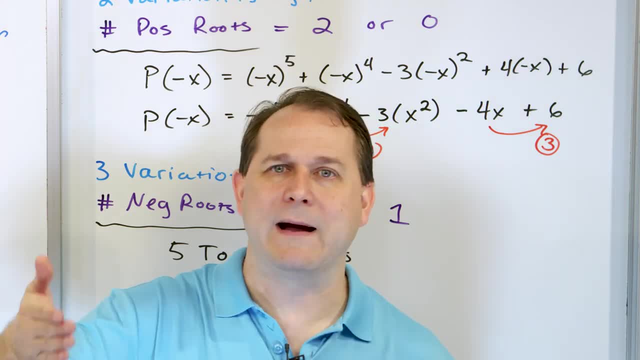 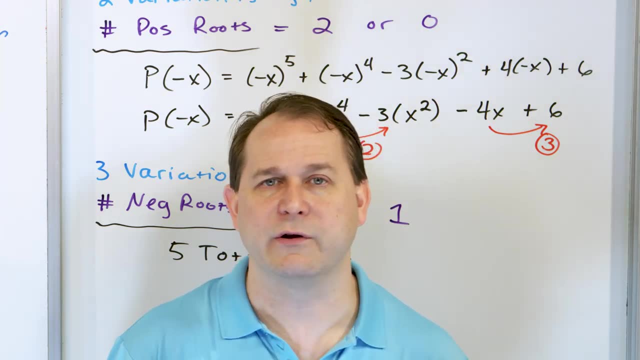 and you can have complex roots right, One plus two i, one minus two i. And we know that those complex roots, if they're there, are always going to be in conjugate pairs because of the conjugate root theorem that we've already learned. 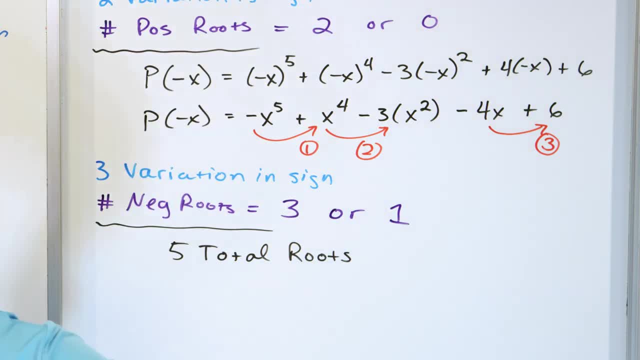 So the best way to do this is to write a table down. So we know we have five total roots and we know that we're going to have some number of positive roots. Right, we know that we're going to have some number of positive roots. 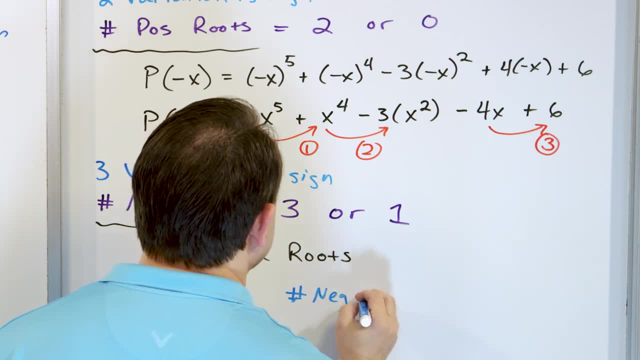 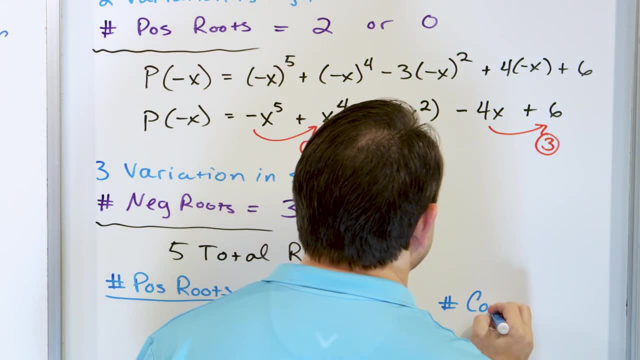 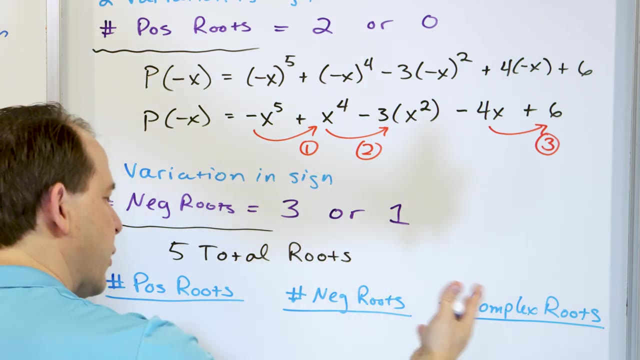 We know we're going to have some number of negative roots, Right. And then we also know that we could have some number of complex roots. And when I say complex roots I'm saying it could be one, i, two, i, you know- pure imaginary. 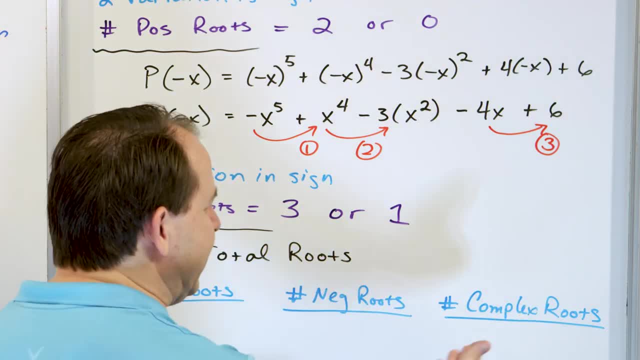 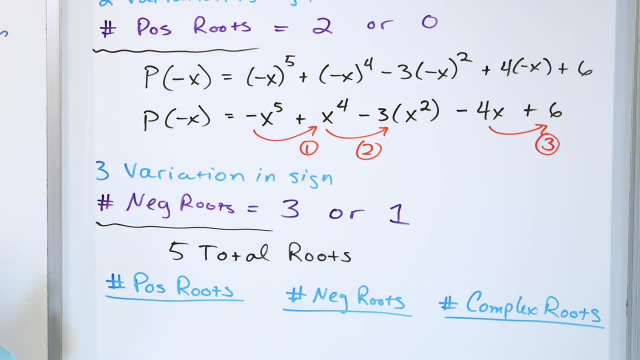 or it could be one minus two, i, one plus two, anything with an imaginary number. Any number is going to go in this column. So what you have to do is you have to take into account all the possibilities here. So the cleanest way to do this is you start. 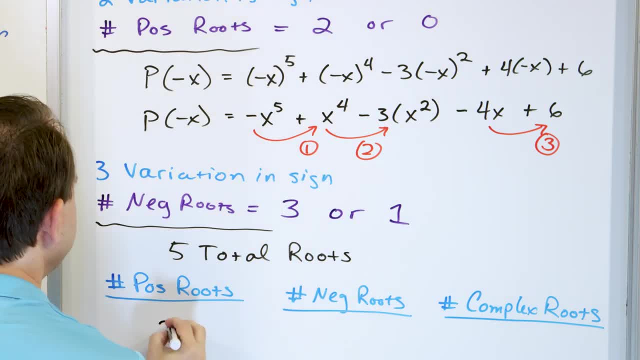 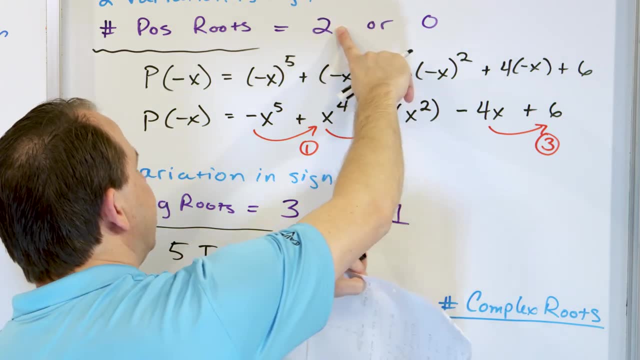 with the positive roots, You could have two roots. I could have two positive roots, But if I lock this down, kind of grab it and lock it down, I could have two roots. but I still have two possibilities of the number of negative roots: three or one. 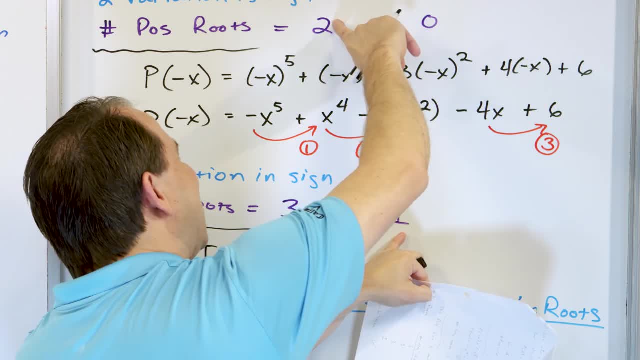 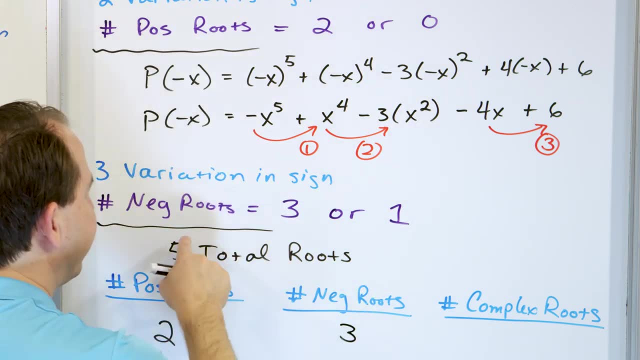 I could have three or one negative roots, while I lock this down saying I have two positive roots, So I could have three negative roots, but if I have two positive and three negative, there's five total roots in this polynomial. Two plus three is five. 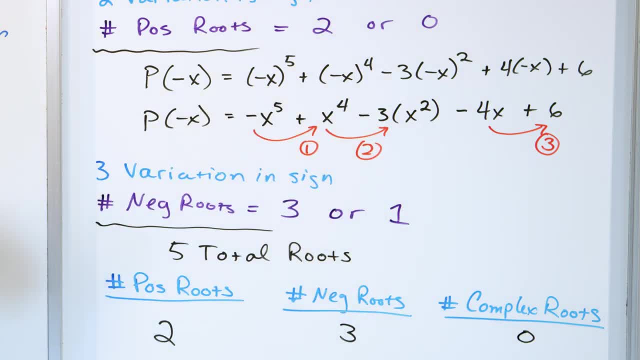 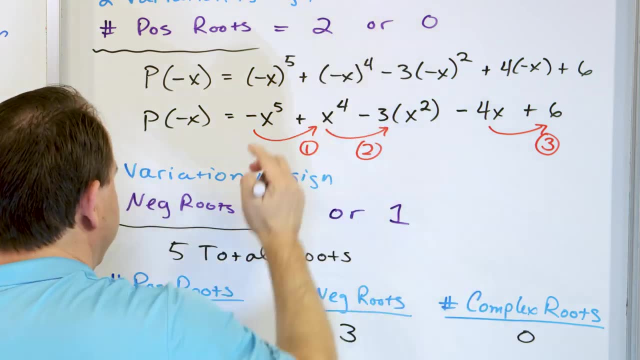 So in that case there would actually be zero complex roots if that were true. Now, if I'm locking this down, this two, I've already done the three. Now I can say: well, what if I had the one negative roots? 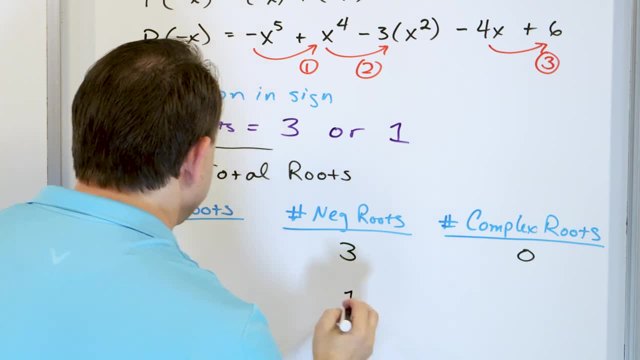 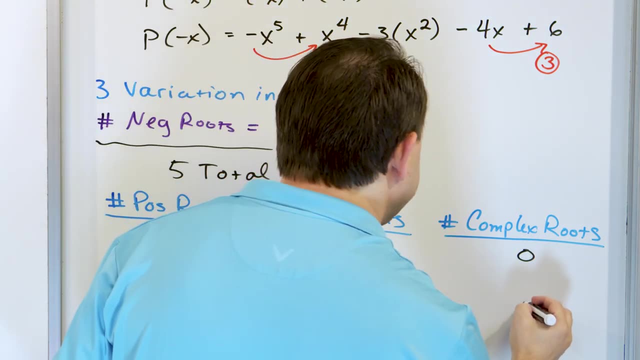 So I would have in that case two positive roots, one negative root. That only gives me three real roots, but I know there has to be five. So there has to be in that case two complex roots, because they have to be three. 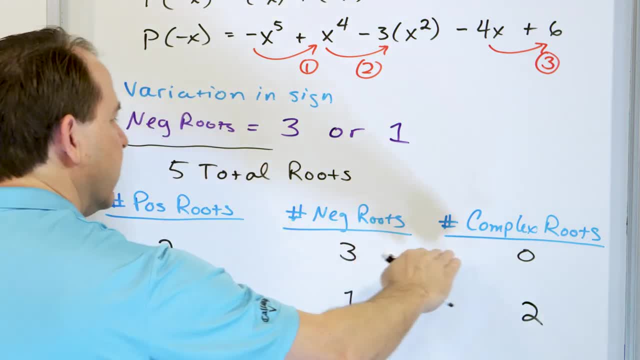 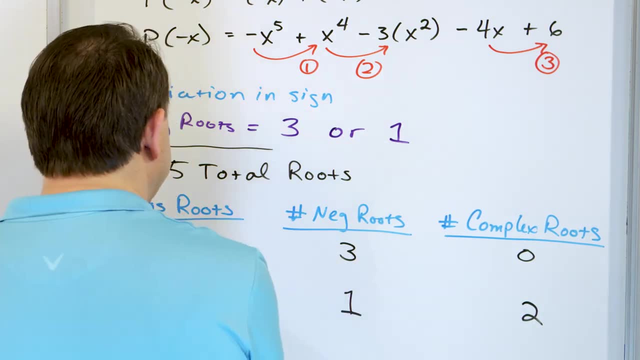 They have to add up to five, right? In this case, it happens that both were real and I didn't have any imaginary roots or complex roots Here in this line. if this were the case, that's true, then I would have two positive, one negative, two complex. 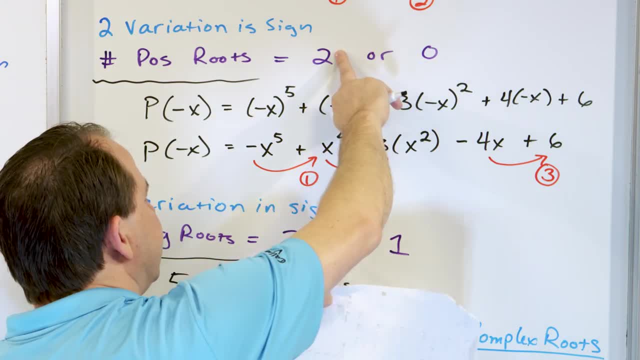 So that was, if I held this constant, I'm done with that. There's no other possibilities here, right? Then I go to zero and say: well, what if I had zero positive roots? Then I could have three or one negative roots. 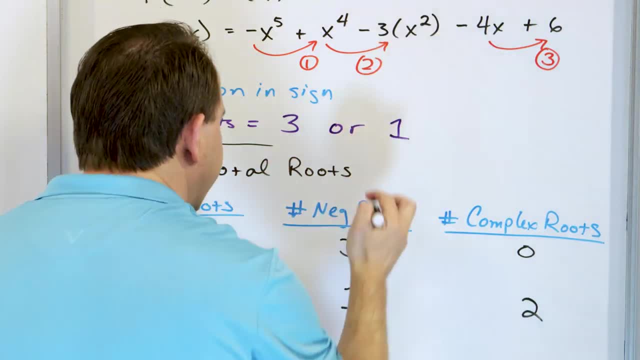 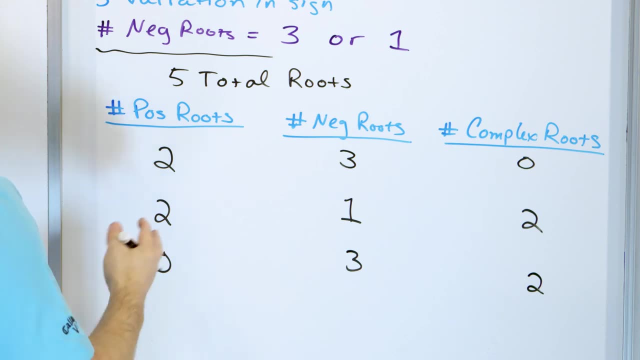 So I could have zero positive. Locking that down, I could have three negatives If those are. If that's the case, then that's only three real roots. I would need again two complex roots to make it equal five. 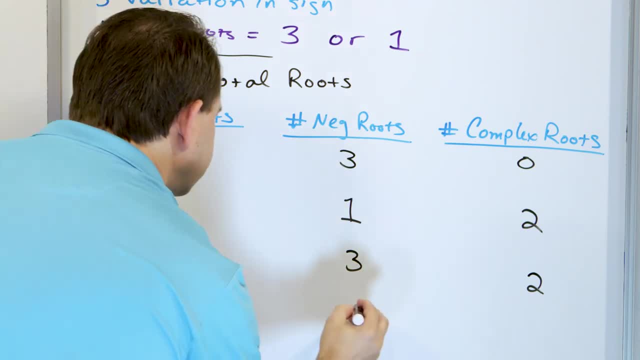 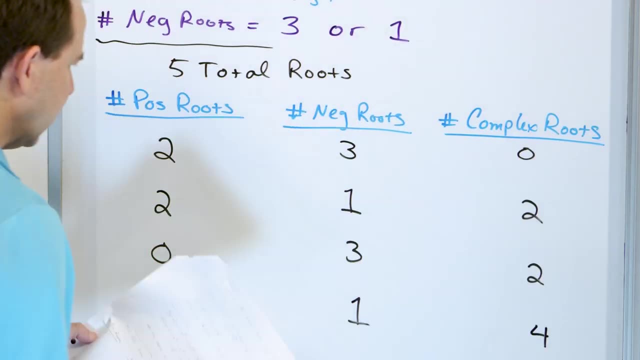 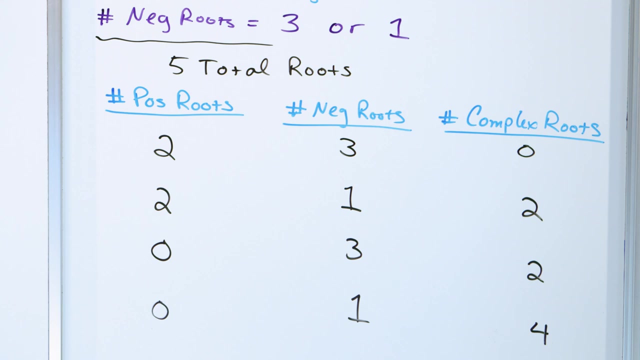 And rounding it out, if I had zero positive and one negative, then that's only one. If you add, there's only one real root. now I would have to have four complex roots. So let me double check myself: 2, 3, 0, 2, 1, 2, 0, 3, 2, 0, 1, 4.. 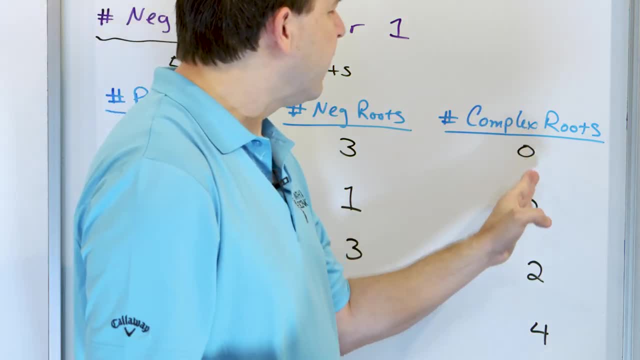 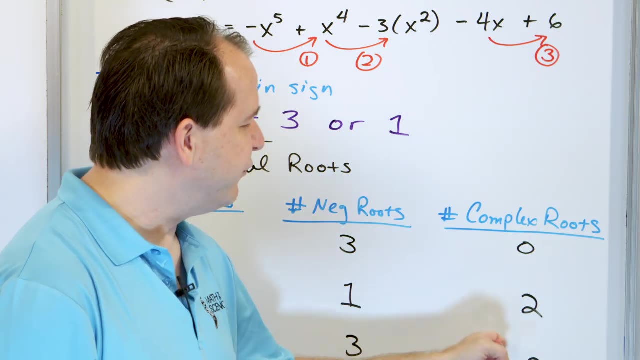 That's correct. So notice a couple of things. The number of in the complex column here is always going to either be zero, meaning there's no complex roots, or it's going to be an even number. See, I had two complex roots, or four. 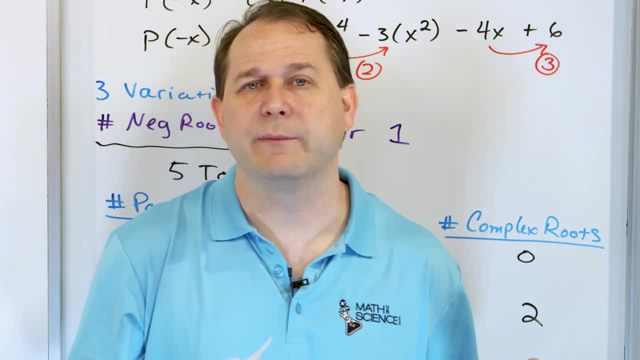 Why do you think it has to be an even number? It's because the conjugate root theorem tells us when we have complex roots they have to come in pairs. You have to have 1 plus 2i and 1 minus 2i. 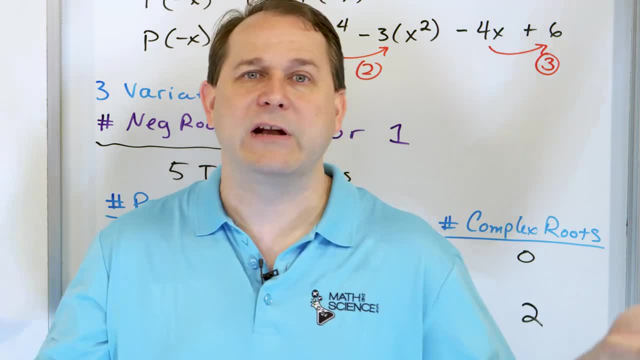 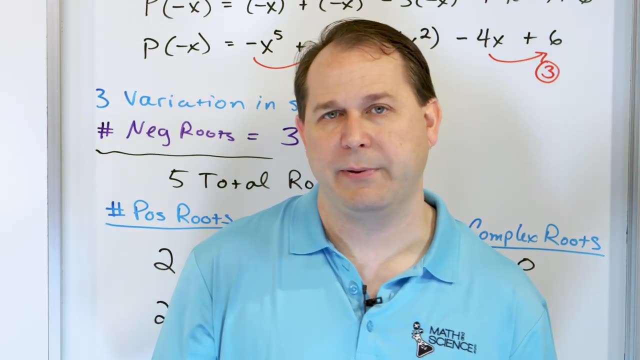 That's 2.. You have to have negative 1 plus 7i. negative 1 minus 7i, That's 2.. So you can never have an odd number of these complex roots, because they always have to come in pairs. 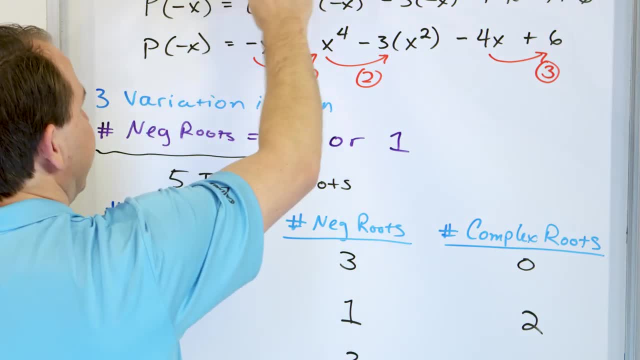 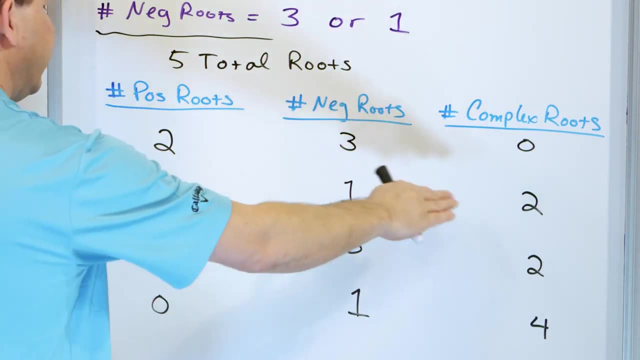 And so you can see that, Even though we don't know what the roots of this equation are, we have built a table. We know there's only really four possibilities: either 2, 3, 0, 2, 1, 2, 0, 3, 2, or 0, 1, 4.. 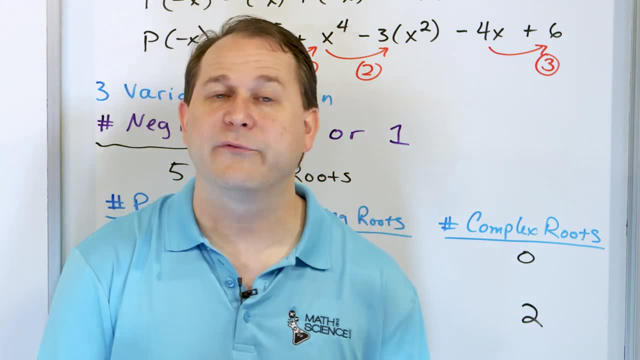 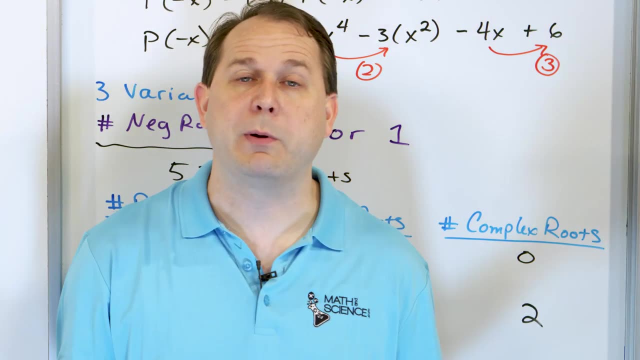 And it's something that is useful in higher level math. sometimes, when you're solving a very complicated problem, Maybe in quantum mechanics or gravity relativity theory or something you have to solve- a large polynomial- Maybe we don't know how to solve that polynomial. 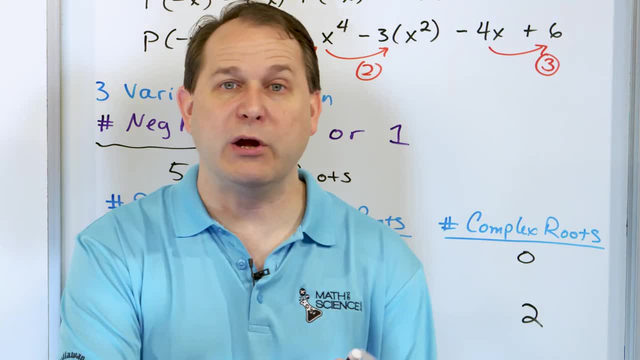 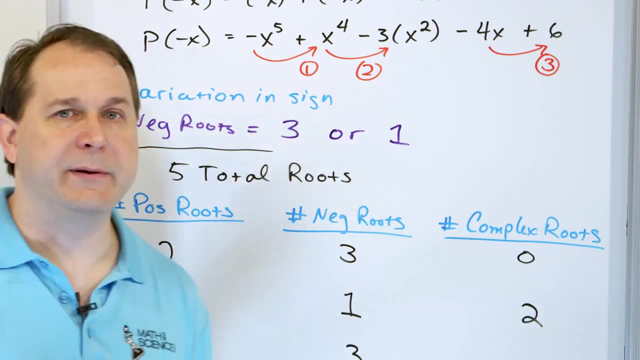 Maybe it's a polynomial so complex- believe me, they do exist- that we don't know how to solve it. But by using something like this, you can figure out what is possible. So you know that there's only four possibilities, and then you can investigate those four possibilities. 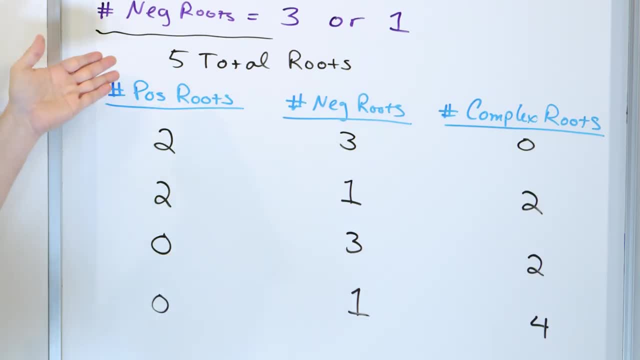 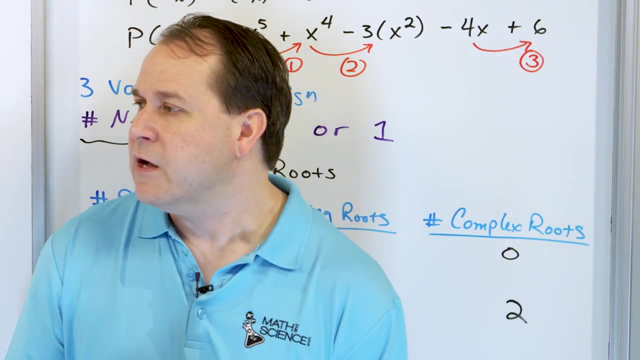 You know, for instance, that you can never have, you know, something that's not in this table as a possible solution set of this polynomial. That's what Descartes' Rule of Sines is all about. So we've done this topic. 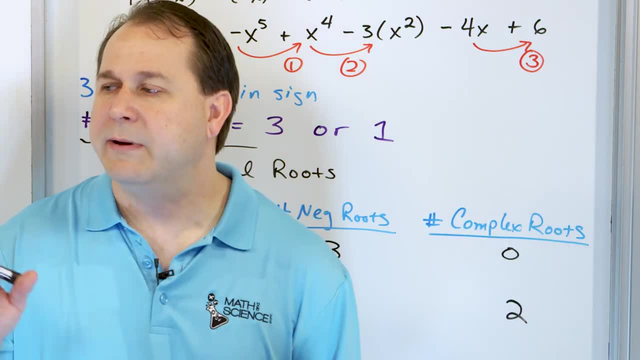 I think it's a good idea if you do this one yourself, just to make sure you understand. But we do have a few more problems, So follow me on to the next lesson. We'll get a little more practice with this Descartes' Rule of Sines. Thank you.